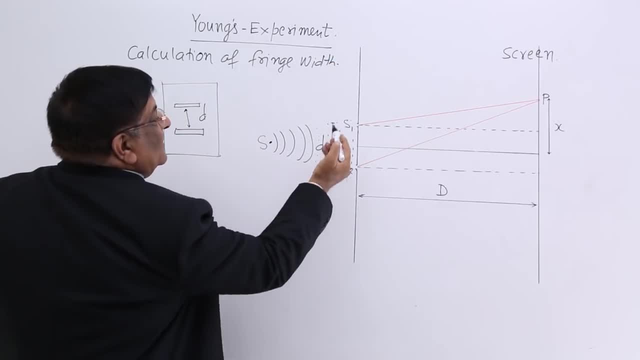 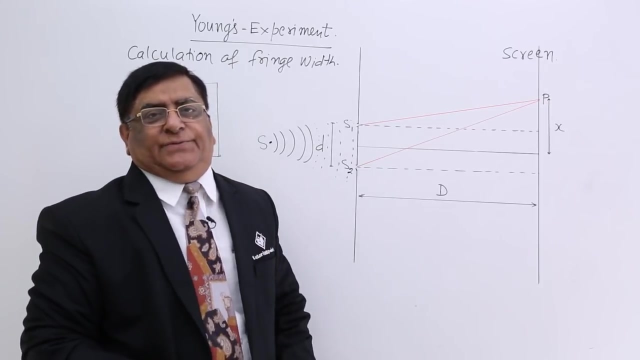 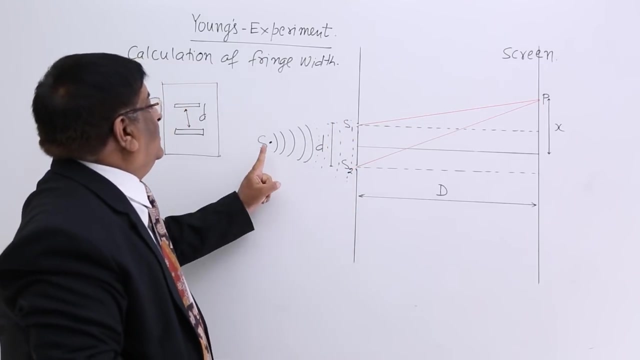 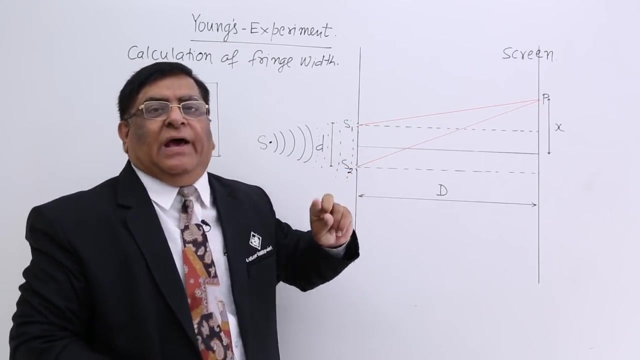 right D cardboard. then at this point one wave front become independent source and at this point, point of wave front become an independent source. So these two secondary sources are made by the wave fronts of this primary source. So the waves generated by this and this will have similar frequency, wavelength and speed. 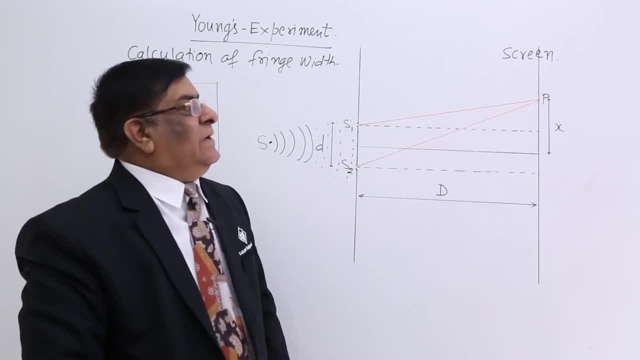 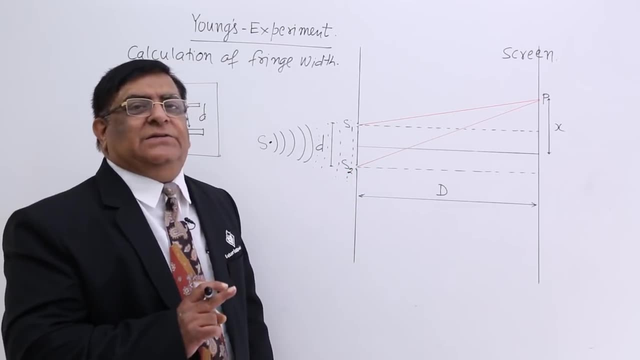 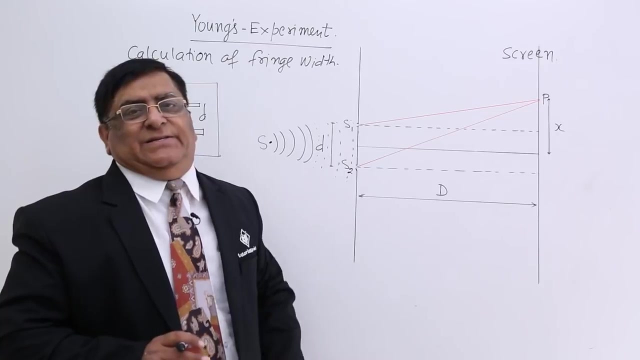 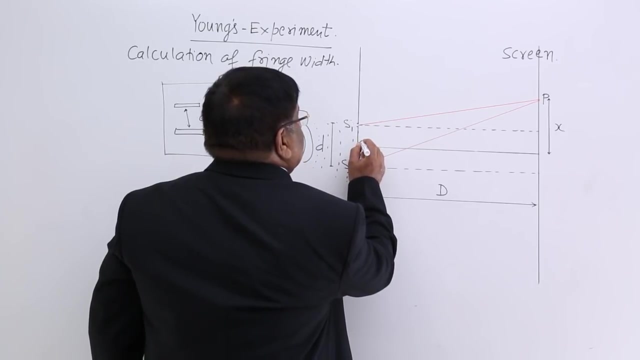 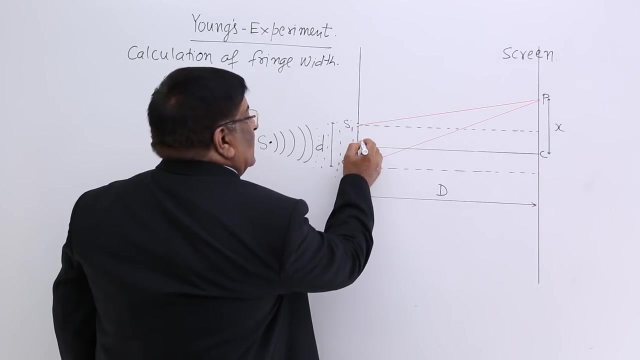 So we will say they are coherent. So these two sources give coherent light. So wherever we get image of the slit, that brightness of the image will be consistent. That is assured. Now, Here this point is, let us say this is a point C, This is a central point O. Now C is such. 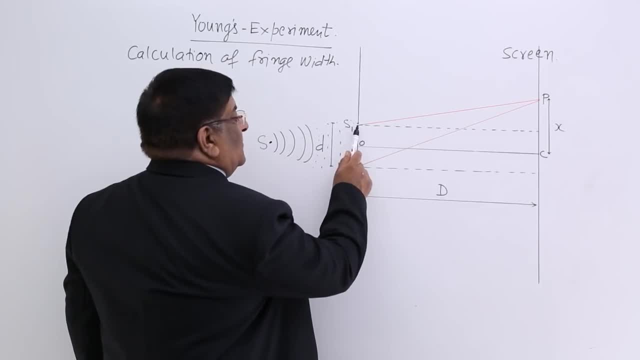 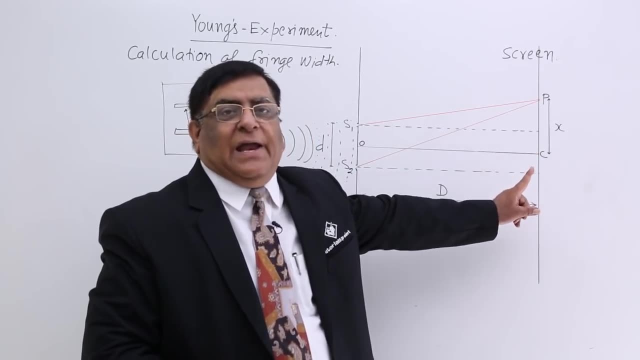 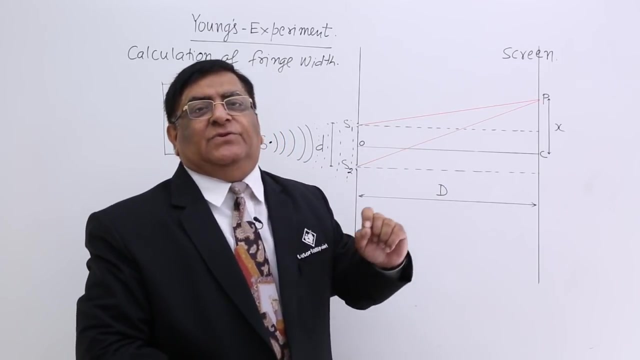 a point which is equidistant from S1 and S2, equidistant from S1 and S2 and at that point the superposition. So So that means this is the constructive superposition. That means from S1 the crest is reaching here. 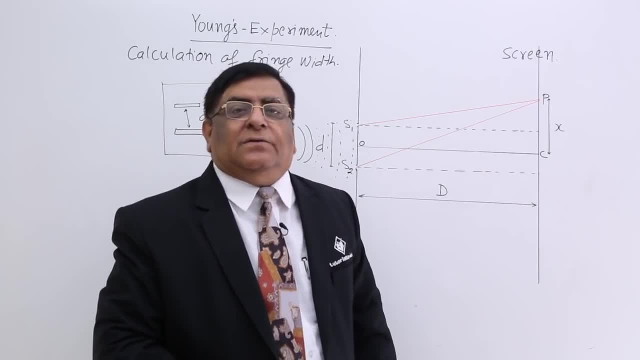 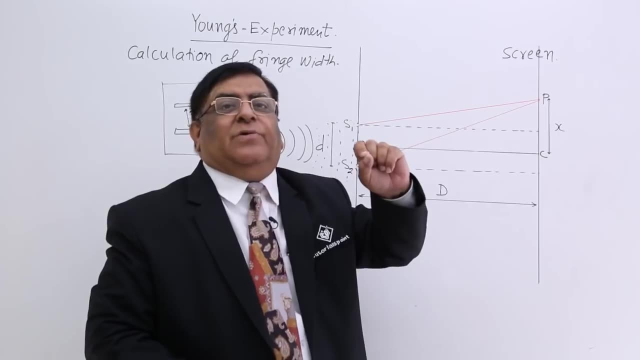 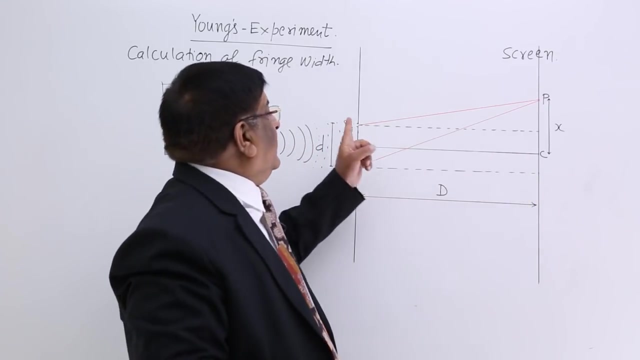 S2 crest is reaching here. That is the point C. We have not chosen the point C. We have chosen that point where brightness is maximum And that is our point C. Why it is maximum there? because it is equidistant from S1 and 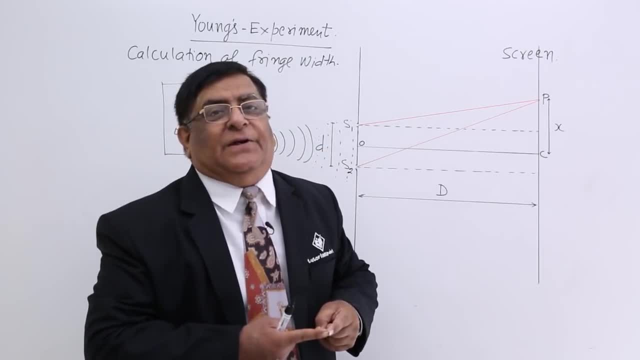 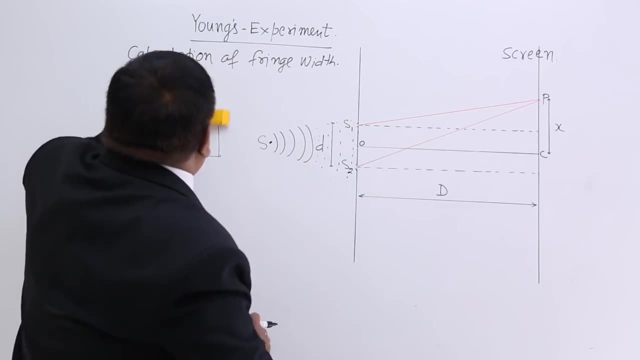 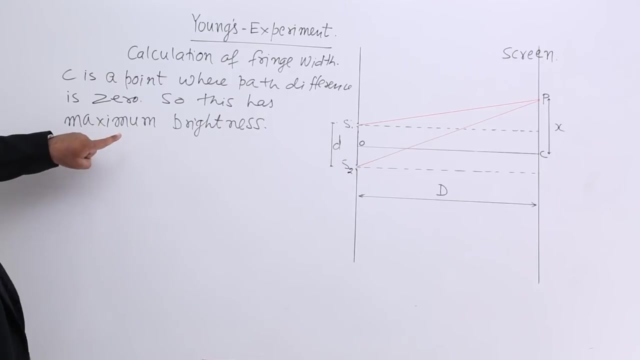 S2.. the waves has got path difference 0. So C is the point. We start from this, the description. So C is such a point. So there is a superposition because the path difference is 0. So C is maximum brightness. We can call it central bright spot. Now, if this is central bright, 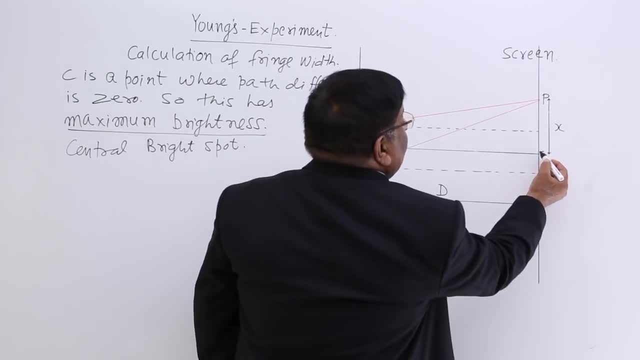 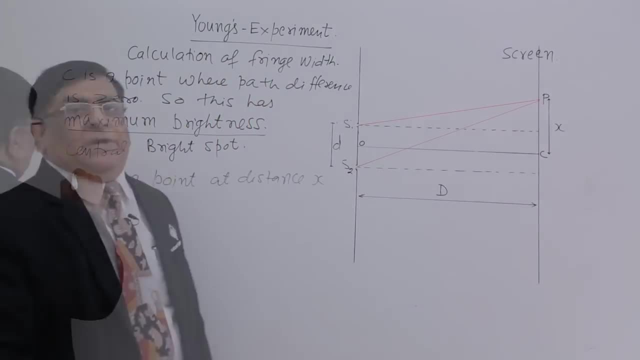 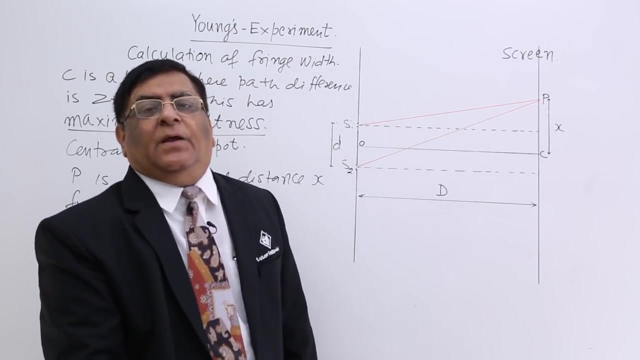 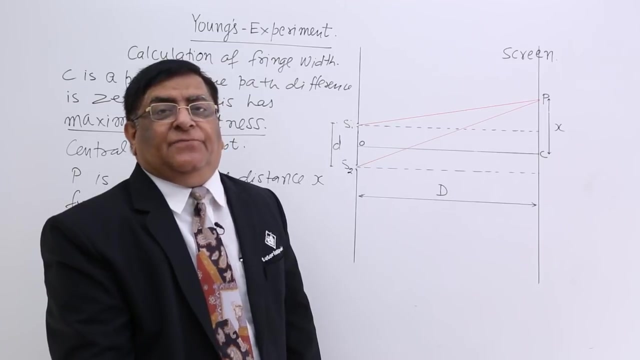 spot. what should be the brightness at point P, which is a distance x from C? P is a point at distance x and we have to find out what is the brightness at this point. How can we find out? We can find out what is the path difference at point P, If we can. 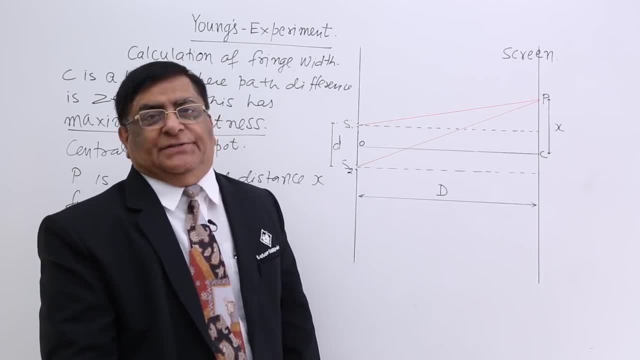 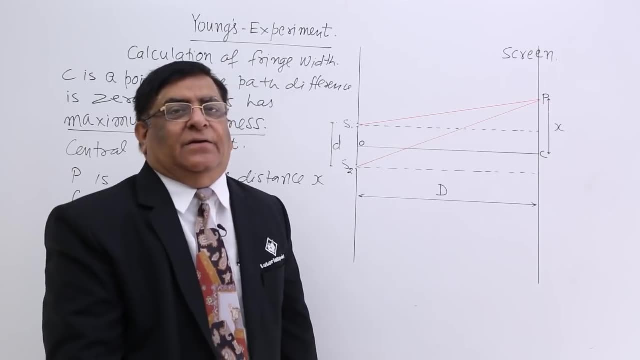 find out the path difference, then we know the conditions. If the path difference is multiple of lambda by 2,, then the brightness is 0. and if the path difference is multiple of 0 or lambda, 2,, lambda, 3,, lambda, then it will be 0. 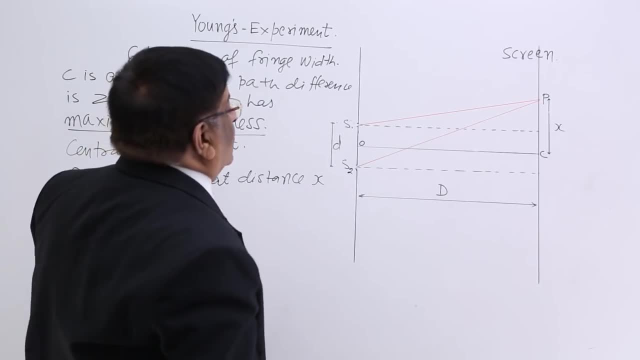 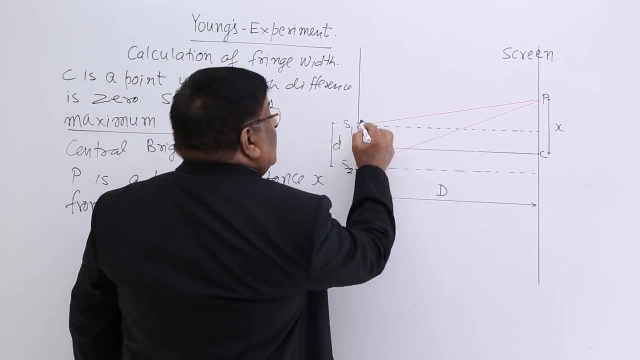 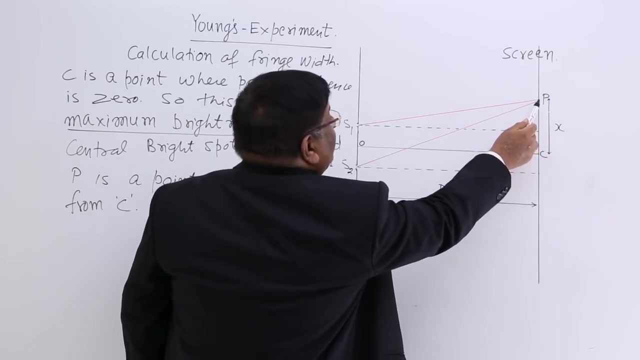 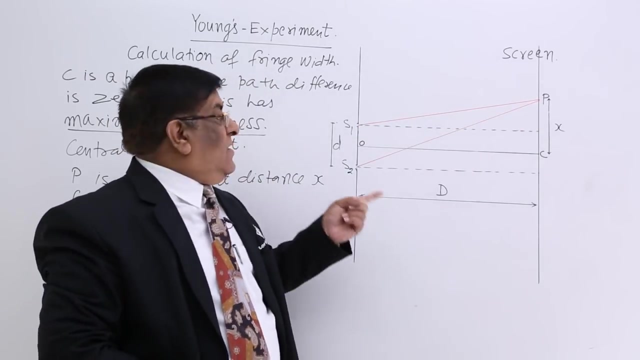 Right, Okay, So how to calculate path difference Now, path difference between what, From S1, the waves are going, This, this, this, this Waves is going, and when it reaches P, what is the length of the path it has travelled? Answer: S1, P. S2 is the source From here. 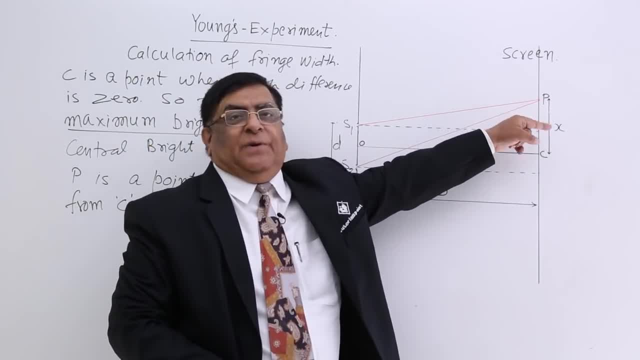 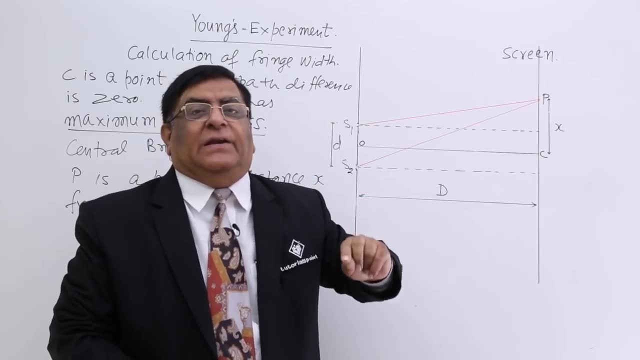 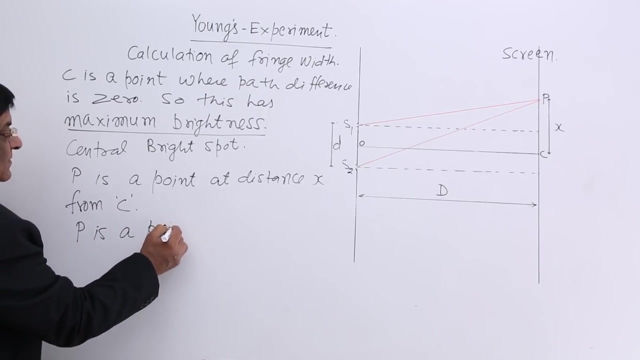 there is a wave travelling and it reaches P. It reaches point P. what is the length of the path it has travelled? S2, P. So what is the difference between the two paths? length? So P is a point at distance x from C. 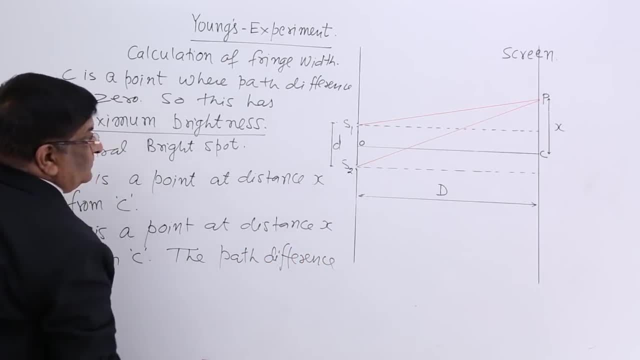 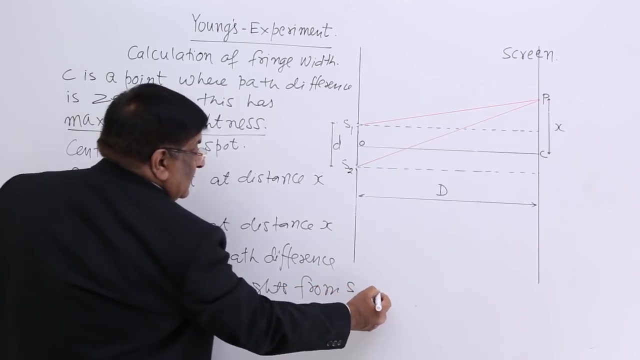 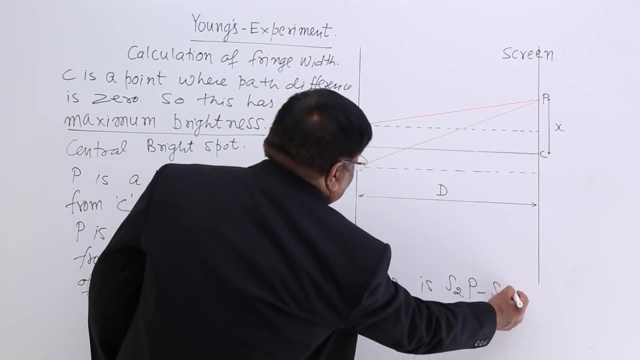 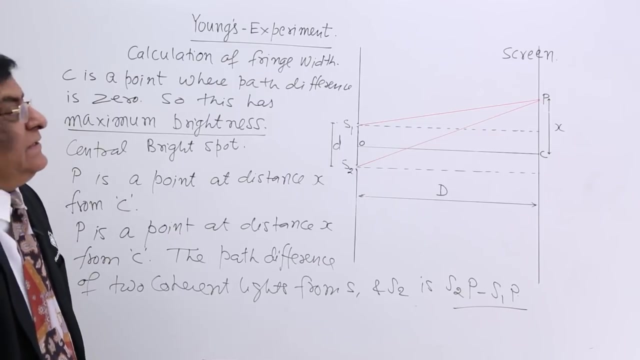 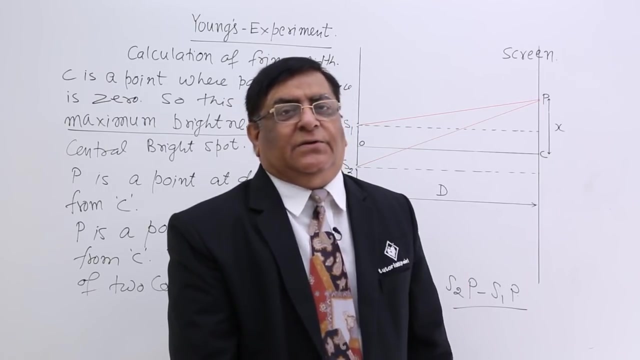 The path difference of two coherent lights from S1 and S2 is S2p-S1p, S2p-S1p. This is the path difference. Now, this path difference, if it fulfills the condition of constructive superposition, then 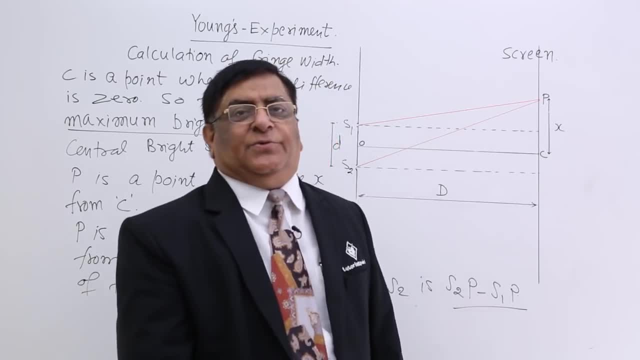 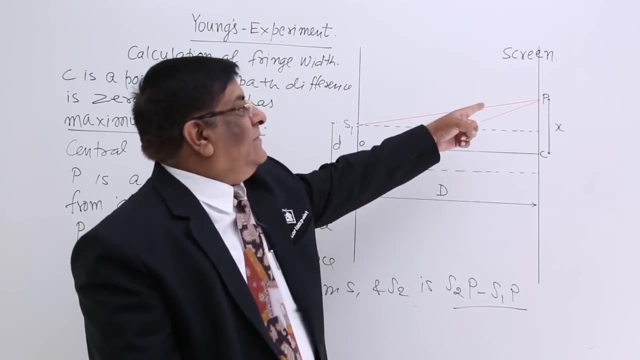 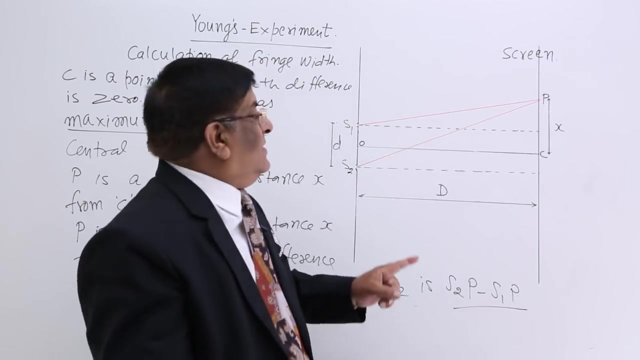 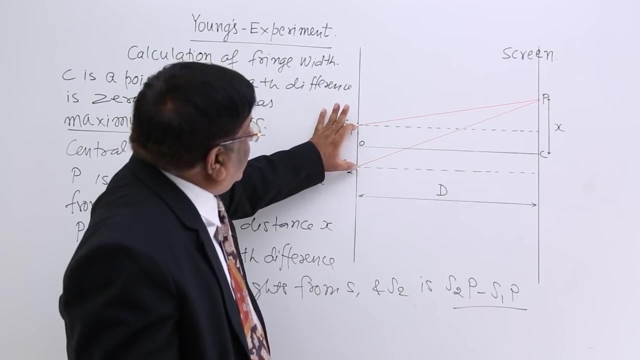 it is bright If it fulfills the condition of destructive superposition, then it is dark, okay. So this S2p-S1p we convert into certain fixed parameters. which are those parameters? that is, the distance between Slit and the screen, the distance between the two slits, d colour of the wave, which 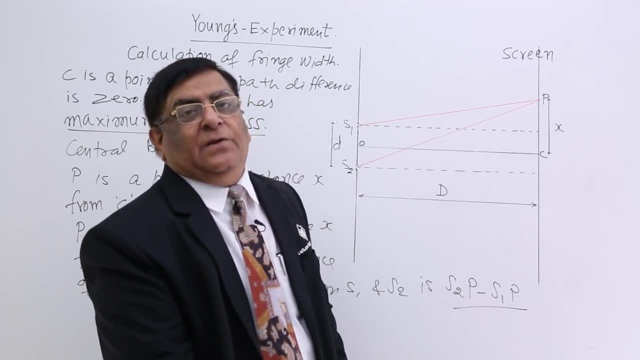 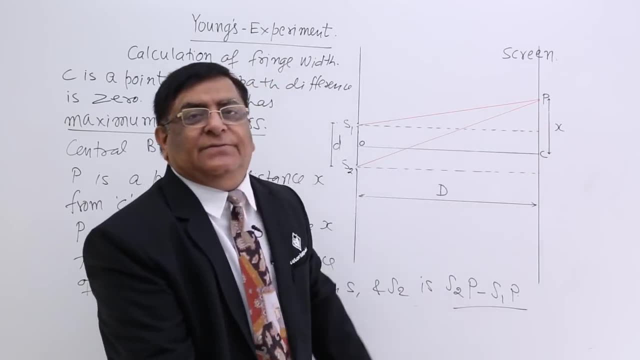 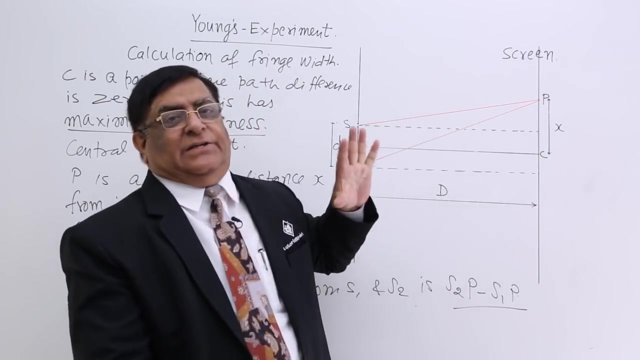 has got a particular wavelength, lambda. So all these three are having effect on this x. So we will translate x into terms of d, d and other things. okay, See how we can do. See how we can do it. What is the path difference? 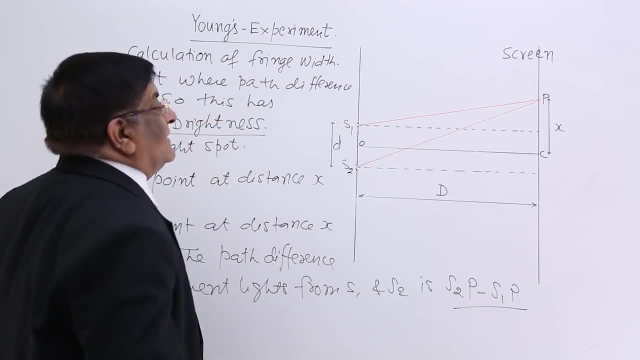 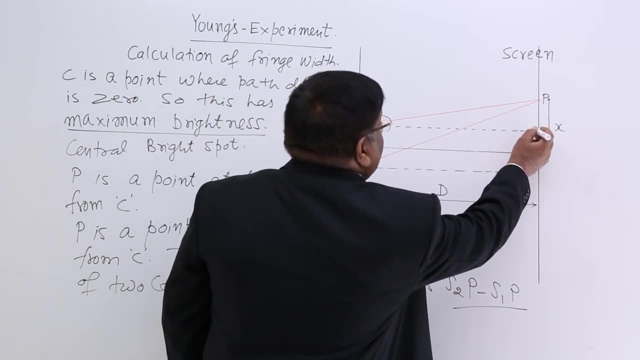 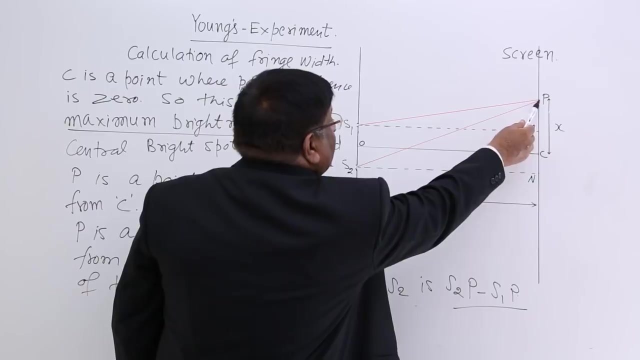 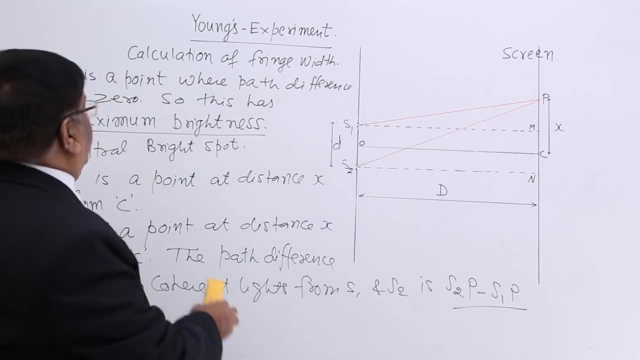 S2p-S1p, and we apply a little bit of energy, a little bit of geometry. Let this point be m and this point be n. S1p can be written as square of S1m plus pm, square, and we start from this point. 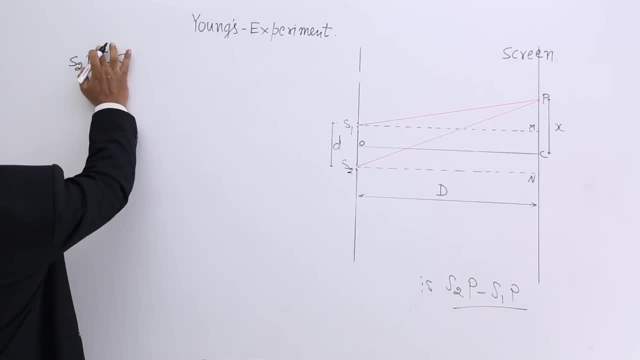 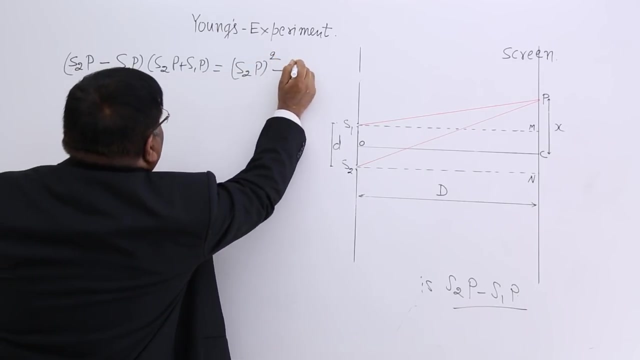 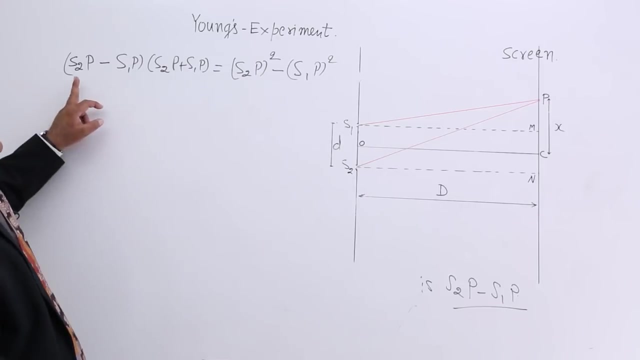 Okay, write an equation this way: S2p minus S1p multiplied by S2p plus S1p is equal to S2p square minus S1p square. a very simple relation of algebra. a square minus b square is a minus b, a plus. 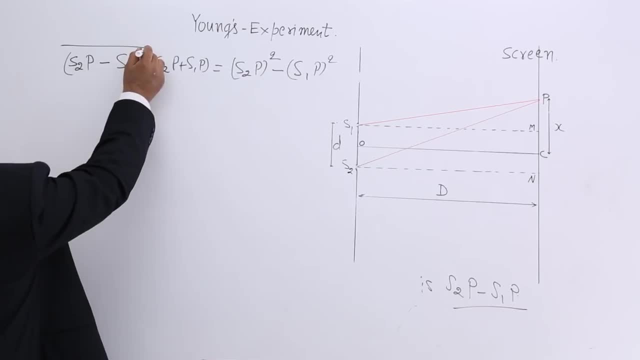 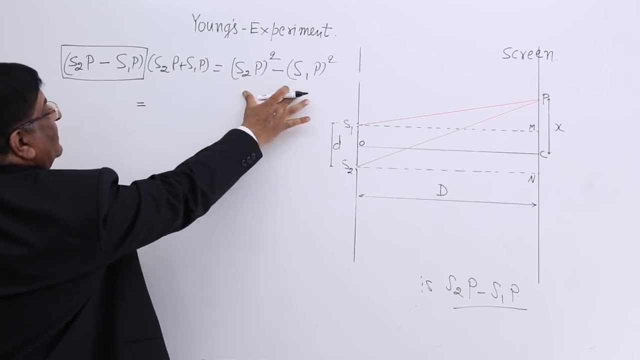 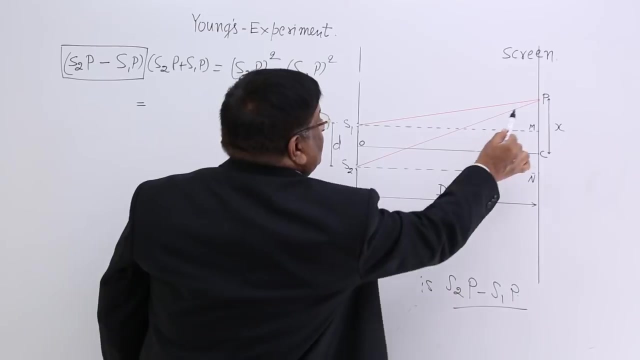 b, this S2p minus S1p, this is the quantity required by S, which is path difference. so we will keep it like this. Now, this is left hand side, this is right hand side, the right hand side we are doing certain operations. that is S2p square, S2p square. we take a triangle, S2p, n, S2, this triangle in. 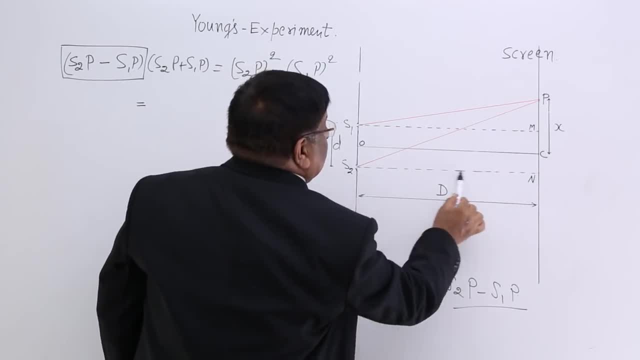 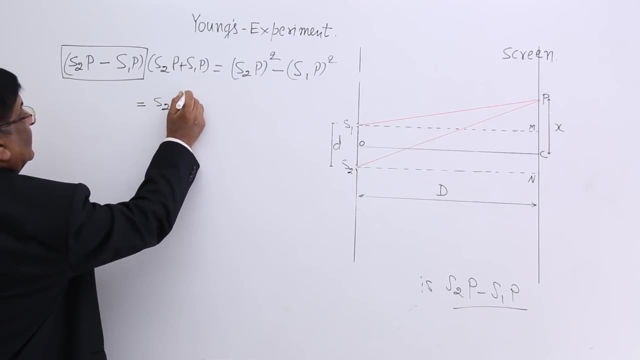 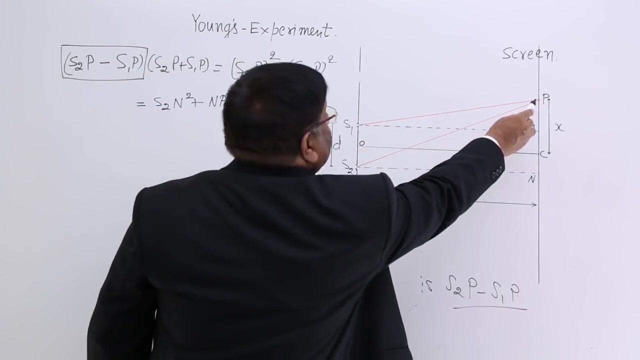 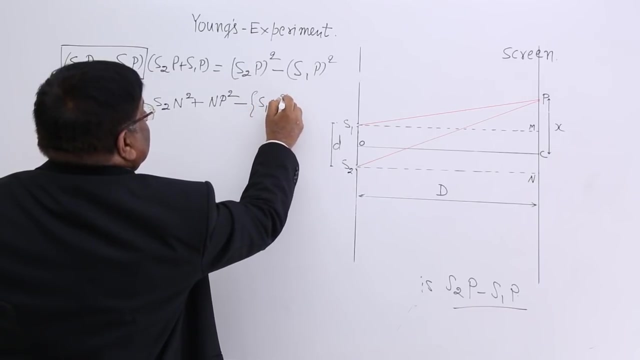 this triangle. So S2p square is square of this plus square of this, so that is S2n square. S2m square plus np square minus S1p square is equal to S1m square. S1m square plus mp square, mp square. 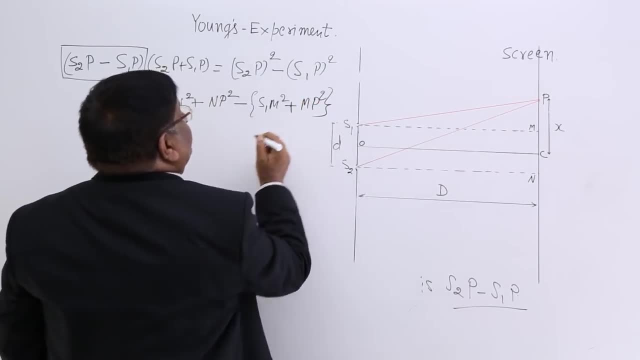 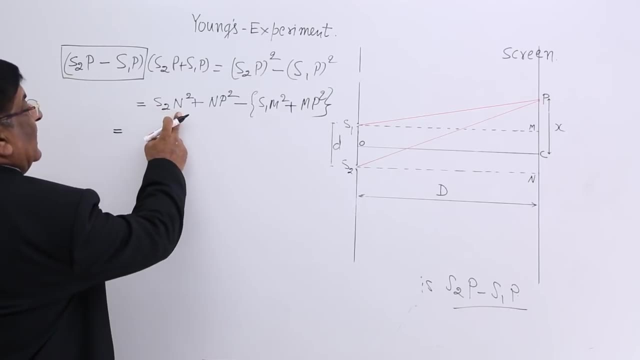 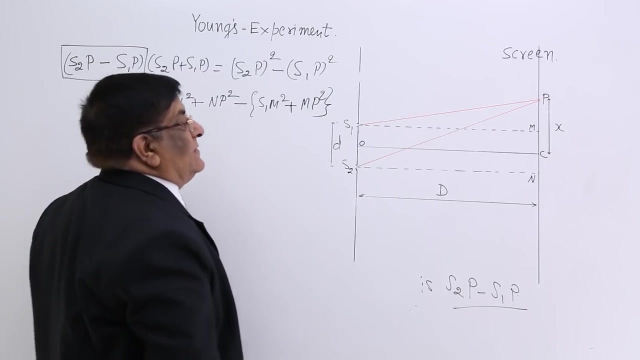 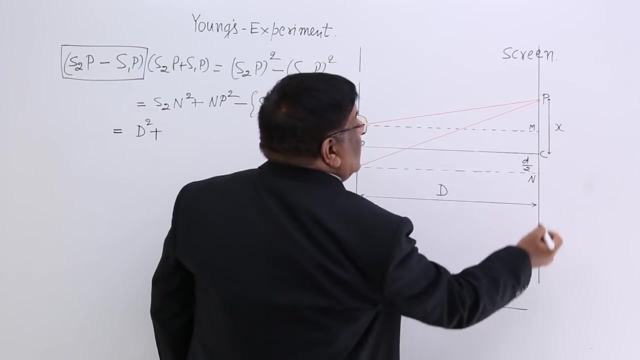 So this is right hand side. Now I convert them in the form of capital D and small d: S2m. S2m is capital D, this is d square plus np. now this width from this to this, this is d by 2, and from this point, 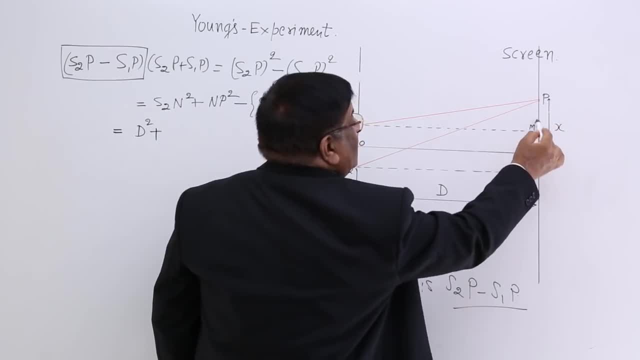 to this point is x, So pn is equal to x plus d by 2.. Now I convert them in the form of capital D and small d: S2m. S2m is capital D, this is d square plus np. Now this width, from this to this, this is d by 2 and from this point to this point is: 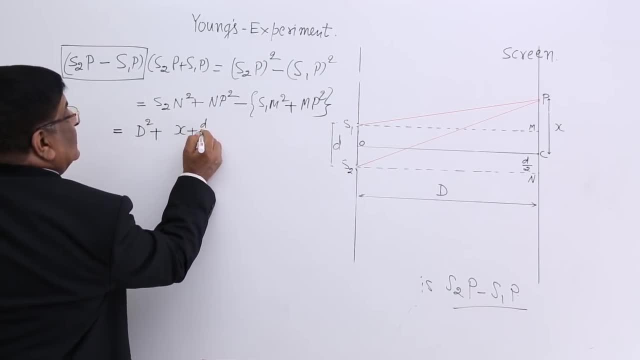 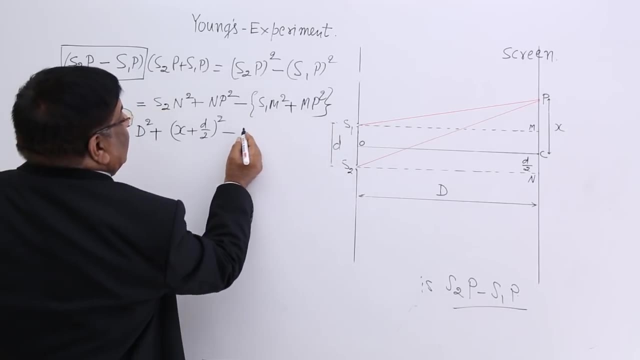 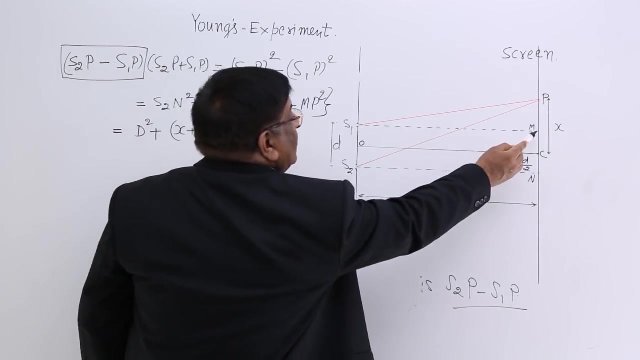 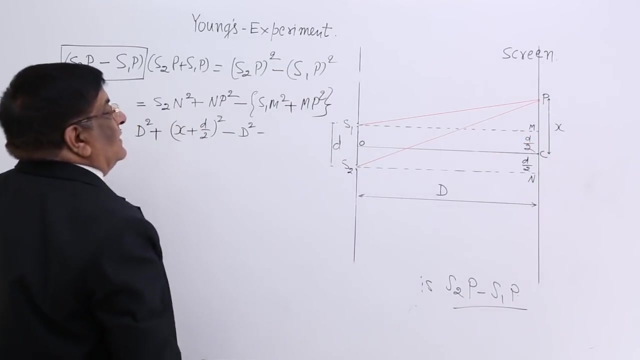 d square, So this is x plus d by 2 square minus S1m. S1m is again d square, minus into plus, minus and mp, mp. this mp is equal to x minus this distance, which is d by 2, so this is x minus. 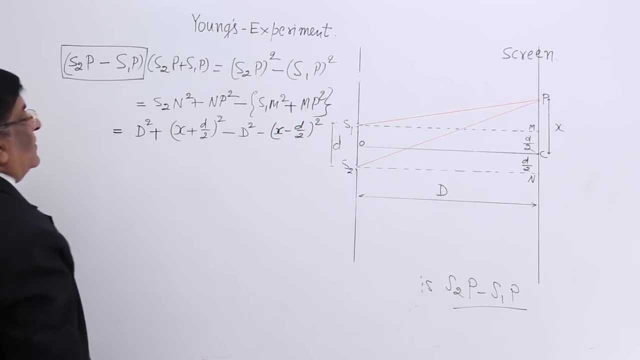 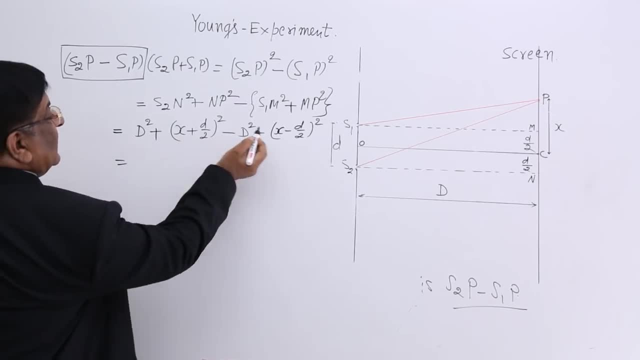 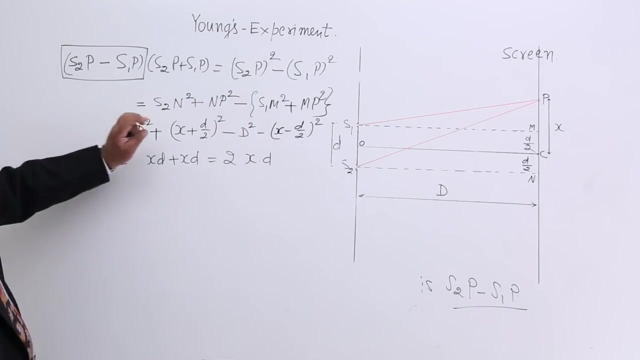 Ok, let us solve this. d square, d square is cancelled. x square, x square is cancelled. d square upon 4. d square upon 4 is cancelled. So what do we get here? xd, and here we get minus into minus, plus xd, So this is equal to 2 xd. this has become like this: 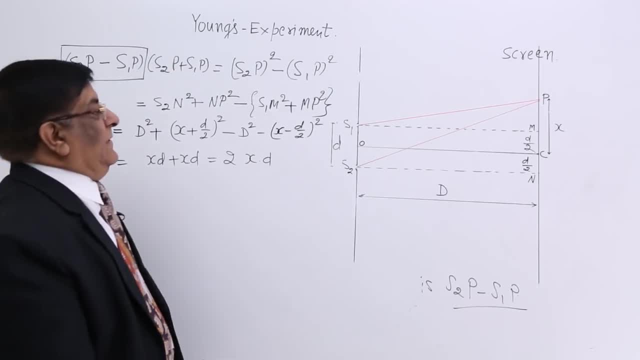 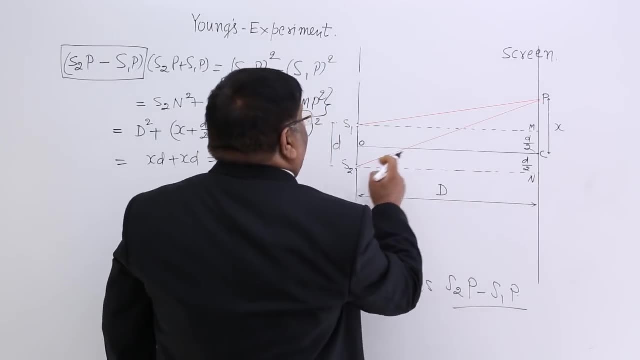 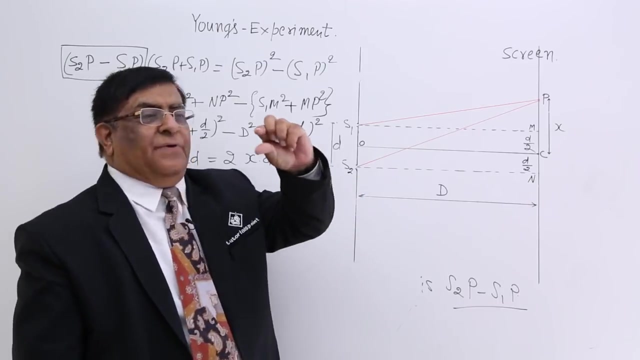 Now come to left hand side: S2p plus S1p plus s1p, s2p plus s1p Now d is the distance between screen and this opening. Practically, when we do this, this distance is very, very small and this distance is very large compared. 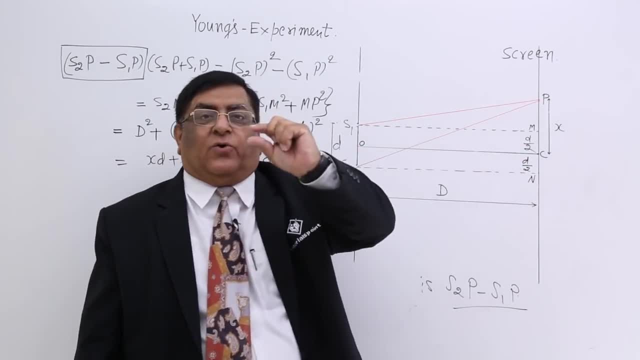 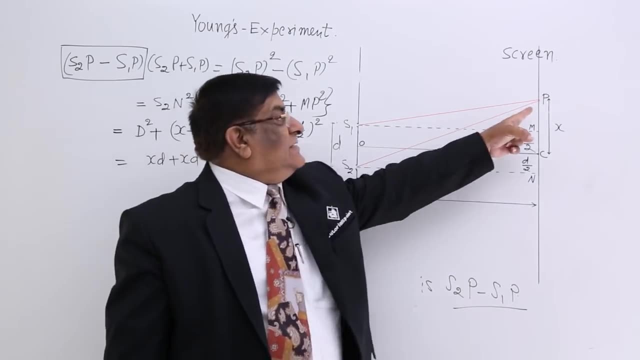 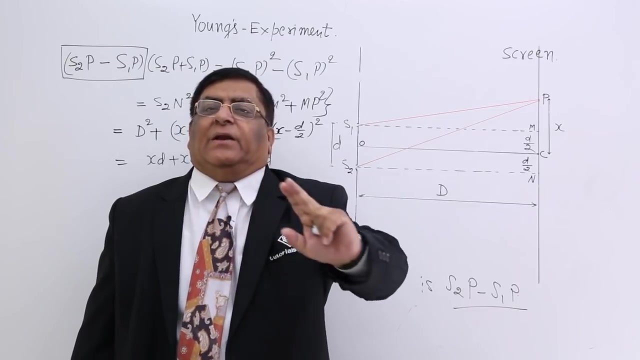 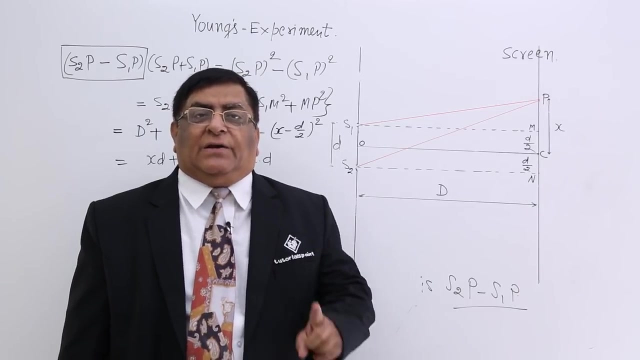 to this distance and this height is also very small. So practically this distance, this distance and this distance when it comes to addition, all these 3 are approximately same. When it comes to difference, difference will be there, but when it comes to addition, like: 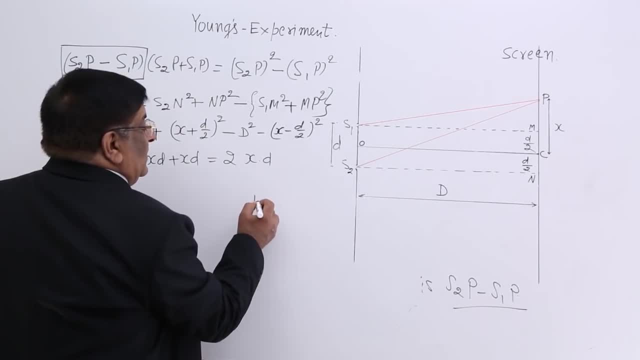 if this distance is equal to, say, 2. 712 mm, this distance is equal to 713 mm. This distance is equal to 712.5 mm. If you do the addition, then it will be 2137 mm. Yes, 2137 mm. 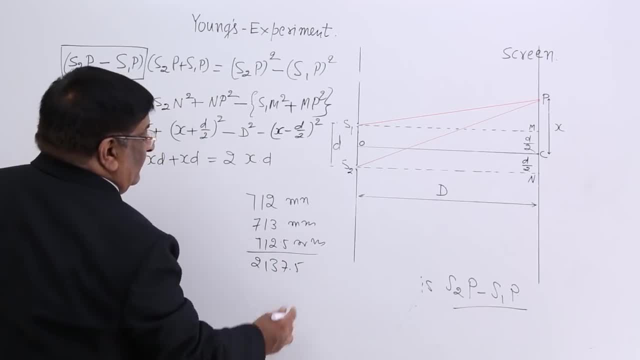 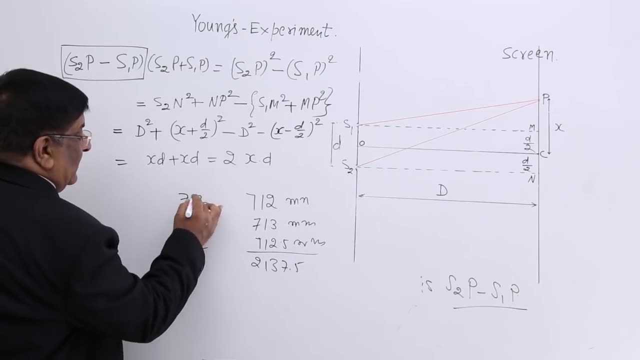 Yes, 37.5. but if you take all 712, 712, 712, then the total will be 2136, which is almost equal. If I write it 2136, what is the error? Answer is: error is only 1.5 out of 2136, that is, 0.005%. 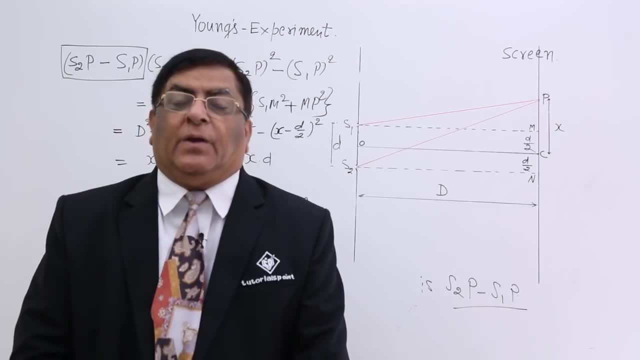 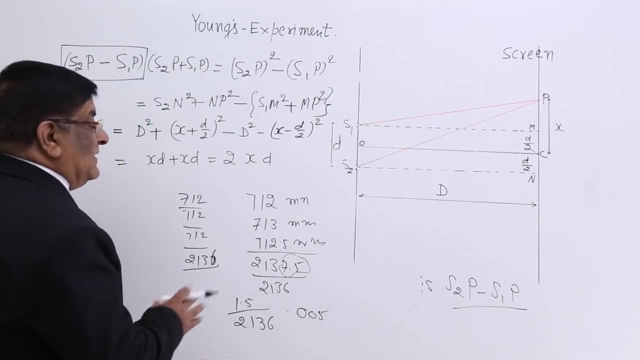 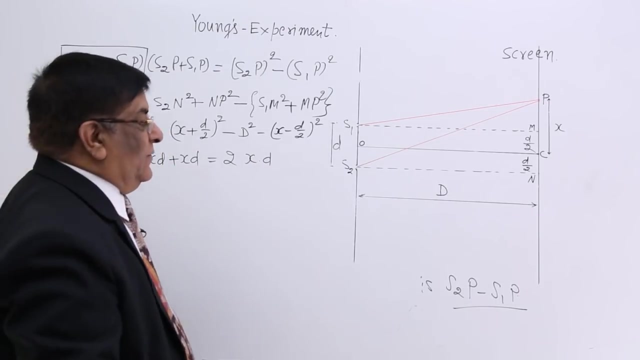 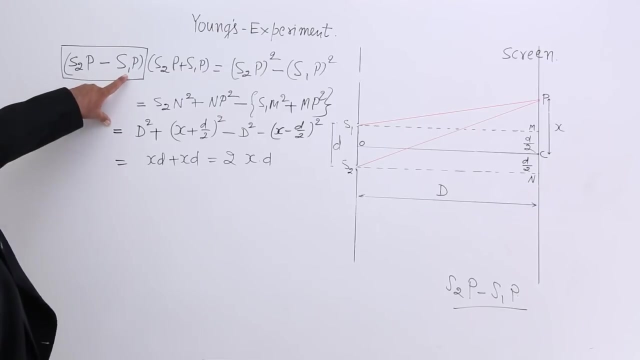 which is negligible. So when we are doing addition then very close quantities we can take at equal, but in the difference we cannot do That we have learnt in class 11th when we were doing measurements. Now S2P, S1P for 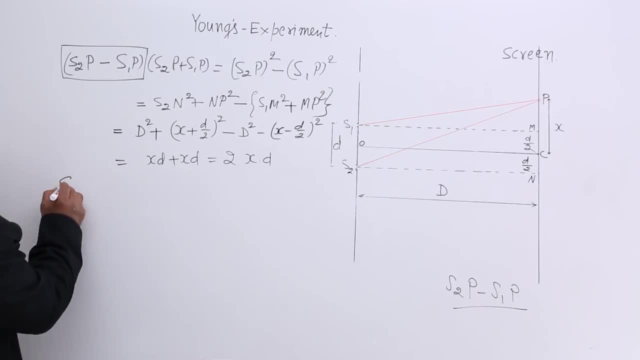 addition purpose. both can be taken: S2P, approximately equal to S1P, approximately equal to D, for addition purpose. Here We can write it as 2D and S2P-S1P. we are not touching because this is our path difference, whose value we need to have is equal to 2XD. So path difference: S2P-S1P path difference. 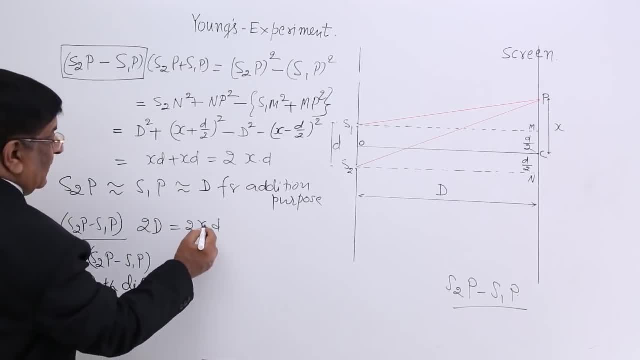 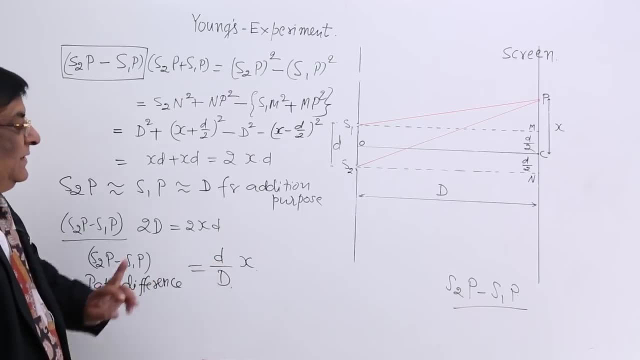 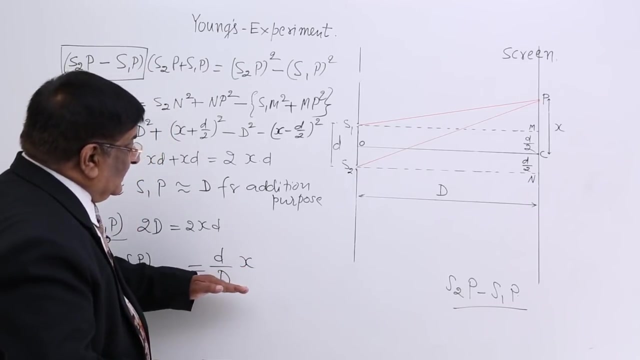 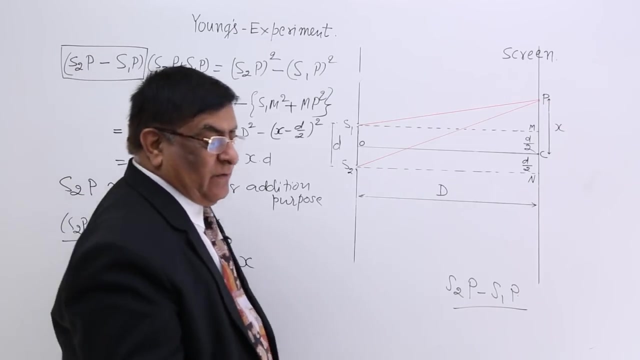 is equal to take it on this side. and what do we get D upon D into X? This is the path difference formula. So path difference: when we are increasing the value of X, path difference goes on increasing. Yes, we can very well understand here both the. 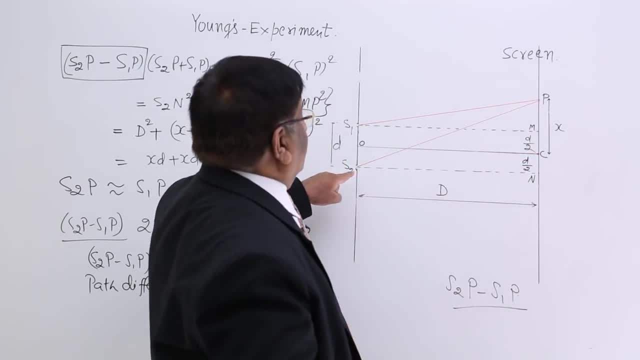 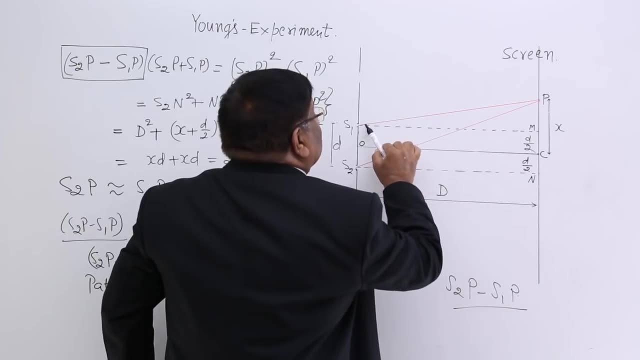 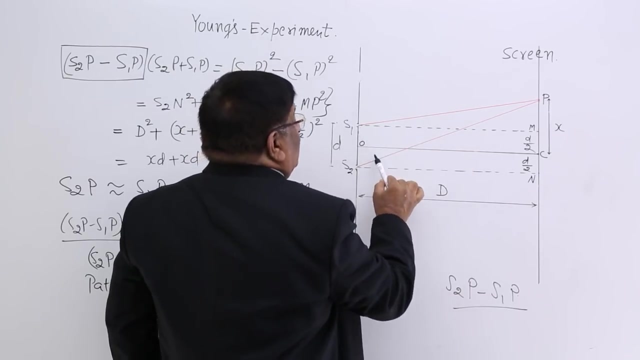 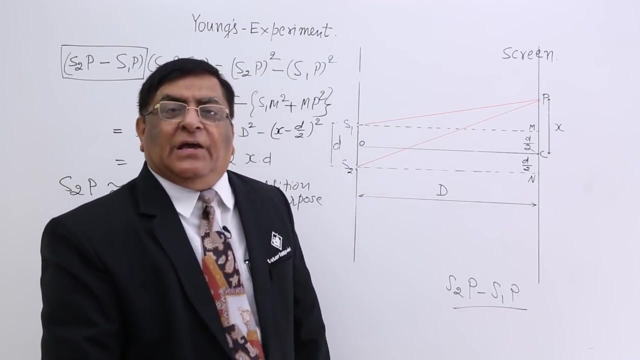 sides will be equal- S1 and this- But when we go up, this side goes on increasing in length and this side also increasing, but this increase less, this increase more and the path difference goes on increasing. Now we know the condition: If this path difference is multiple of half, 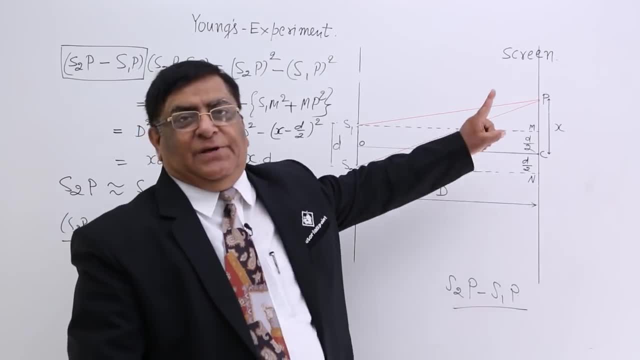 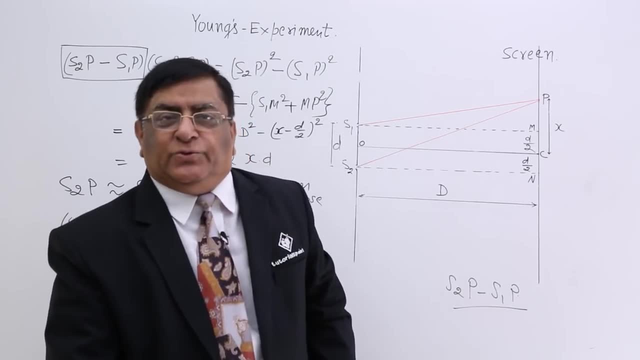 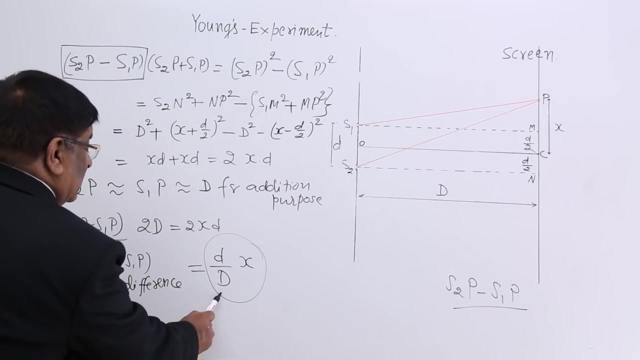 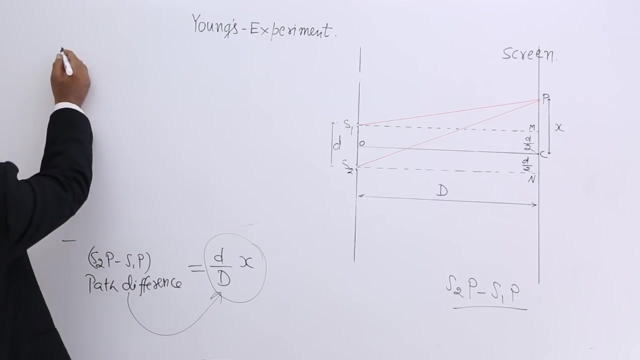 lambda, Then It will be a dark point, and if it is multiple of lambda, then it will be a constructive superposition. and once we have got this formula of path difference, we will use this as path difference and proceed further. Point P: P is a bright point. 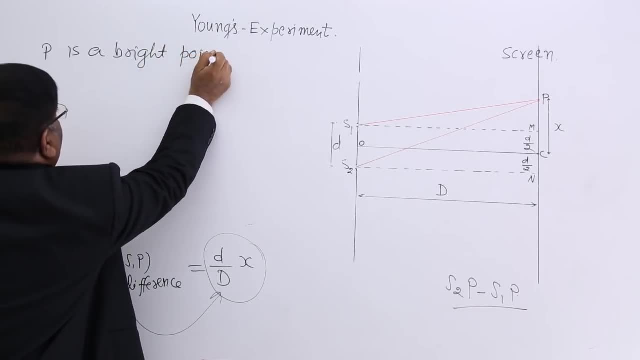 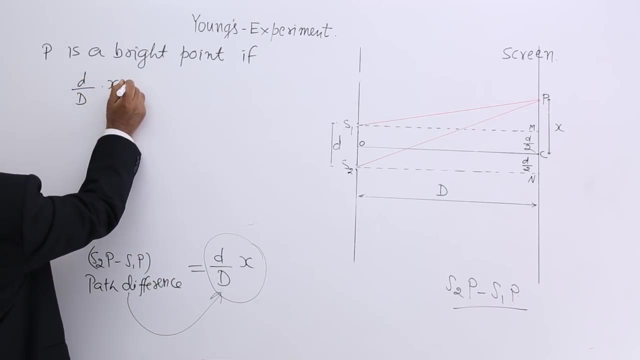 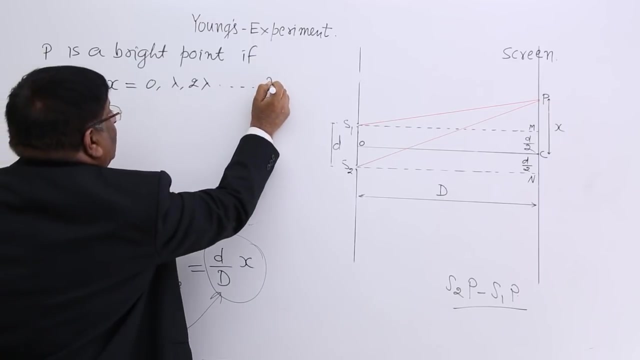 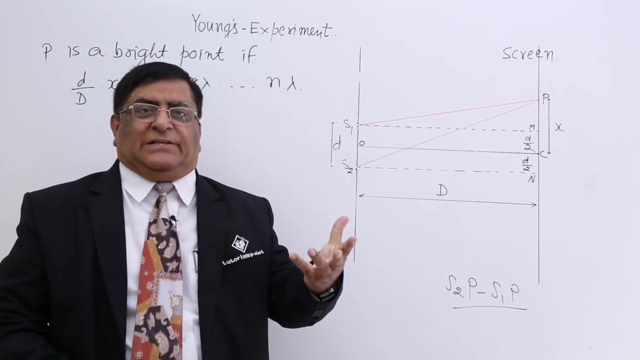 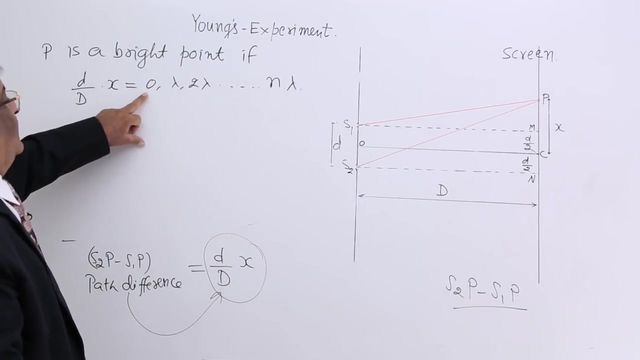 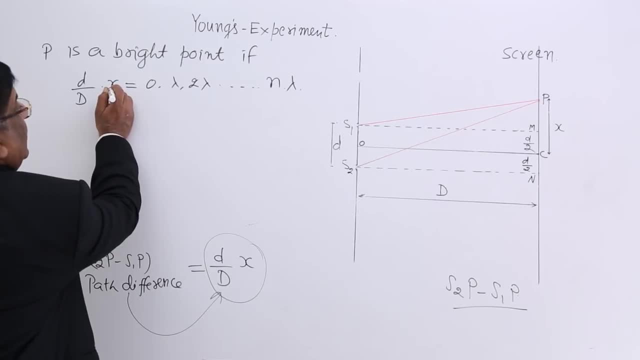 by thisミou, do not З impresaßуby private power. So what should be value of X? X, the transfer d by D on this side? so this will be n lambda d by D, This n. 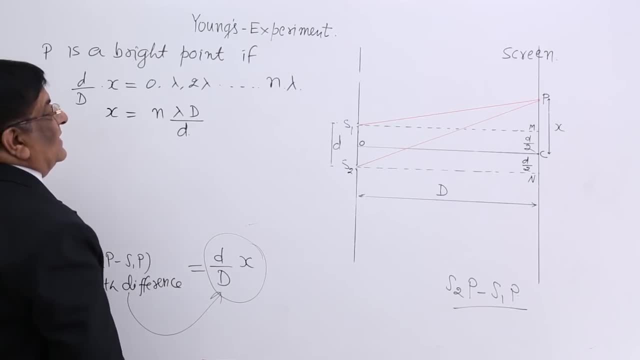 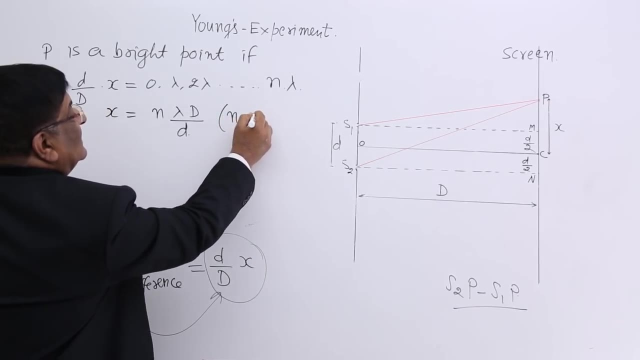 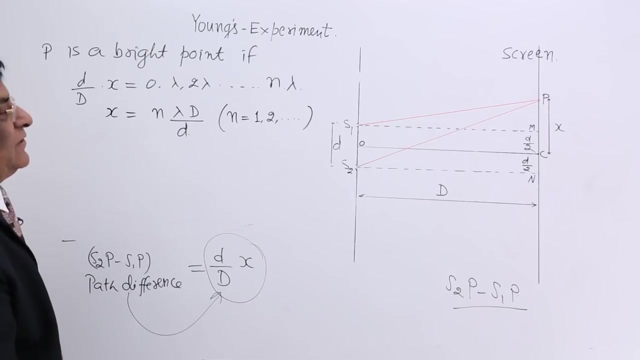 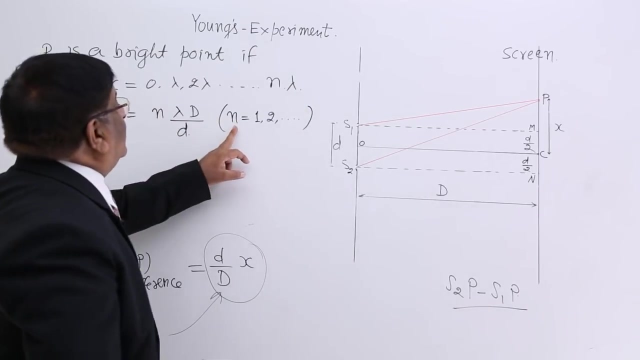 n is integral number, and from where should we start it? So we recommend that here we should start with: n is equal to 1,, 2,, 3,, 4 and not from 0. Why? Because when we say n is equal to 1,, 1,, 1. 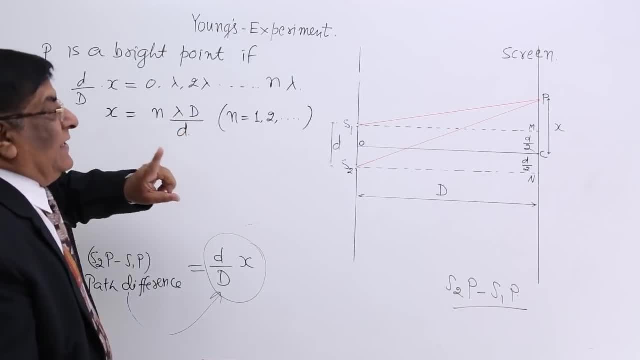 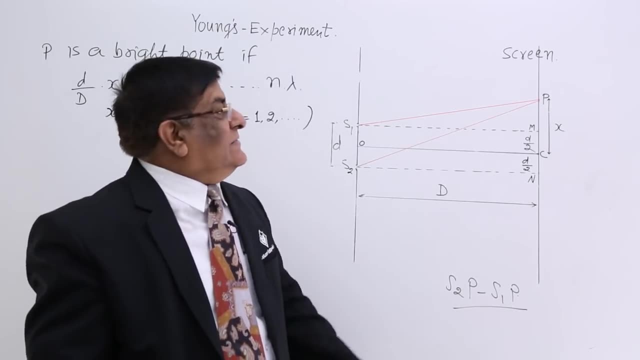 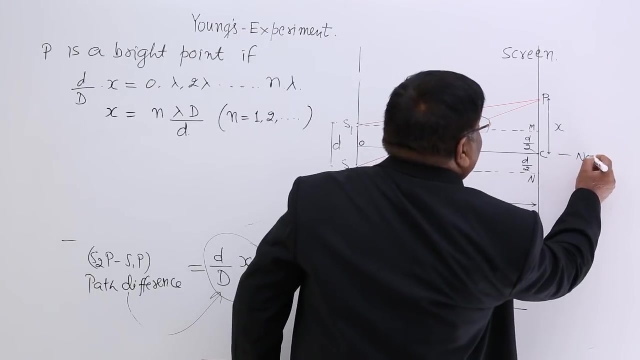 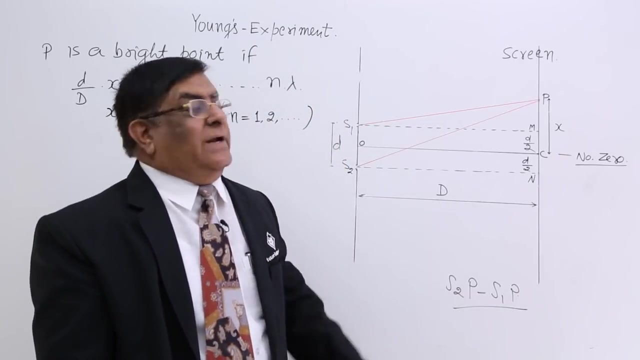 then it is lambda d by d and we get bright fringe number 1.. Where is the path? difference: 0?. Answer: at the central bright. What is the number of this fringe? So this has number 0. We do not give it any number, This is number 0. Then after this, the first bright will be. 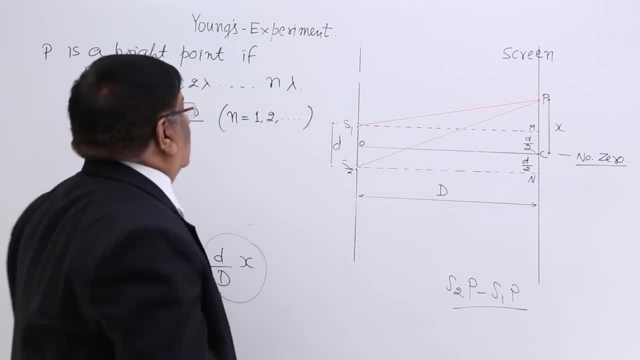 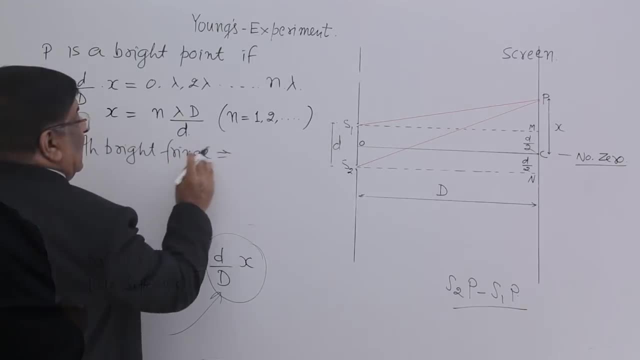 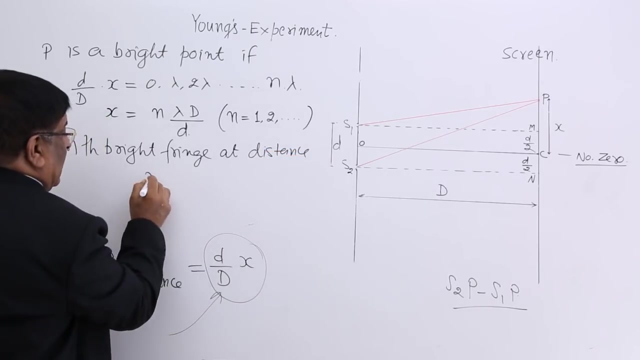 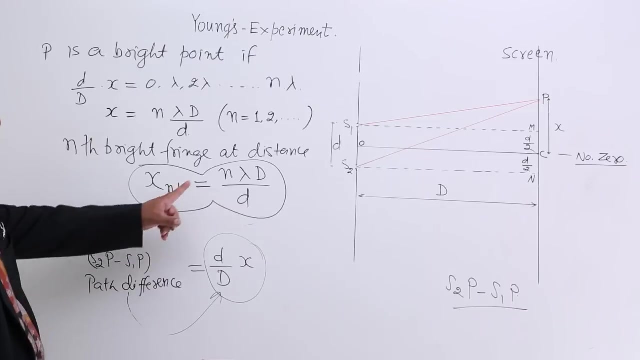 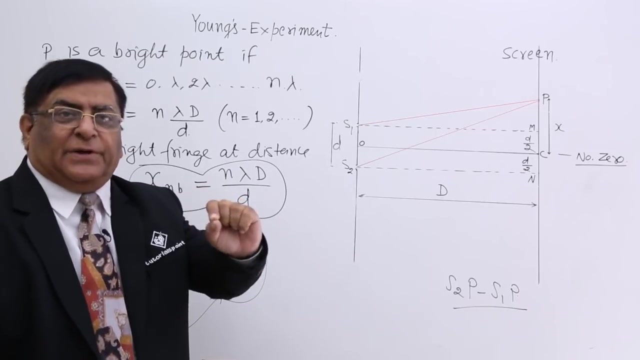 made where path difference will be 1 lambda. So here, how do we get 1 lambda? Answer: if n is equal to 1.. nth bright fringe at distance x: n bright which is equal to n lambda d by d. This is formula of nth bright fringe. If I ask you, I am using orange light which has got a particular lambda. 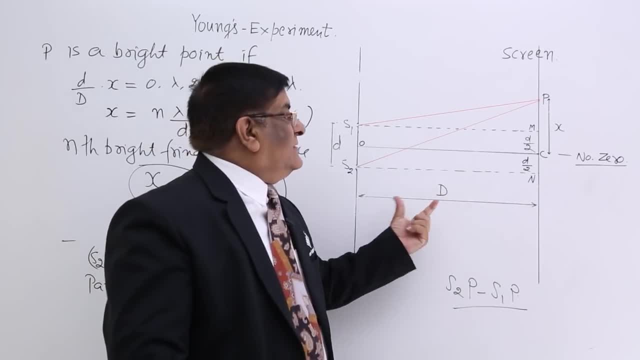 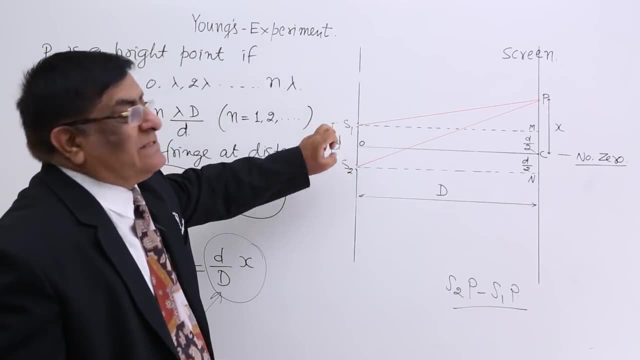 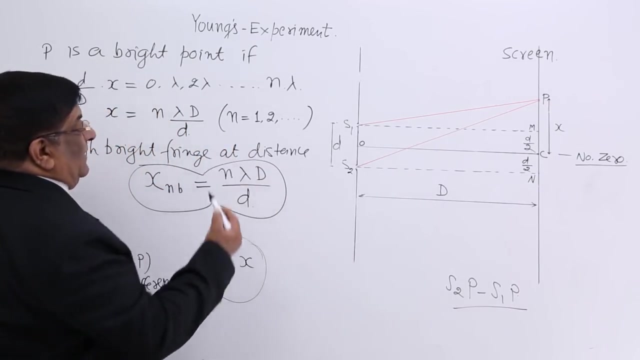 Ok, The screen is at a distance 1 meter right, 1000 millimeter. This distance is equal to 4 millimeter. You got the d, you got the d, you got the lambda. Now I am asking you where. 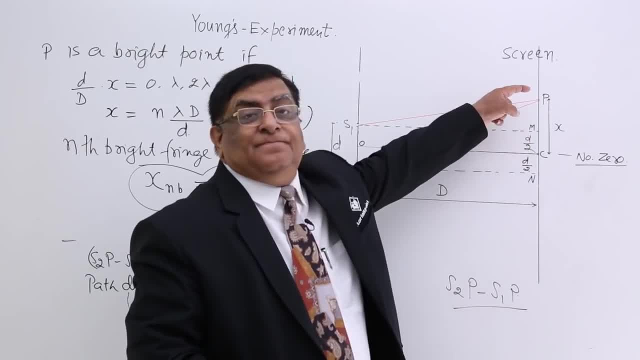 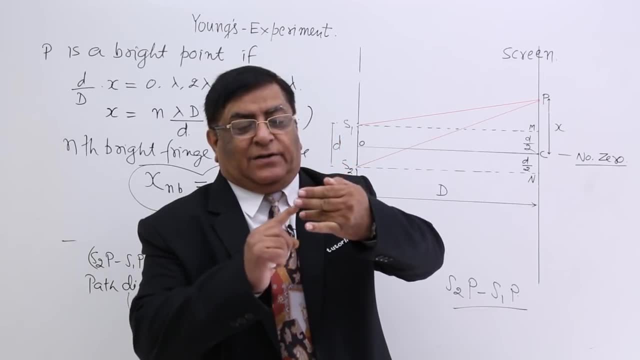 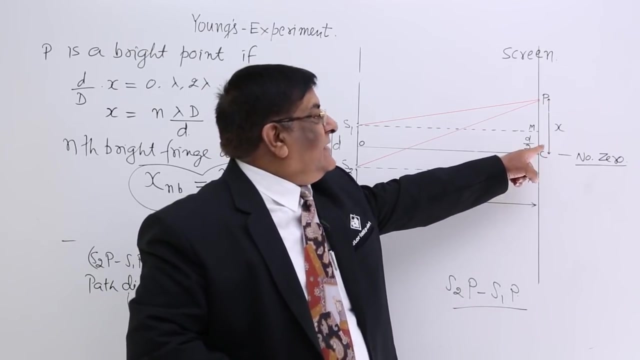 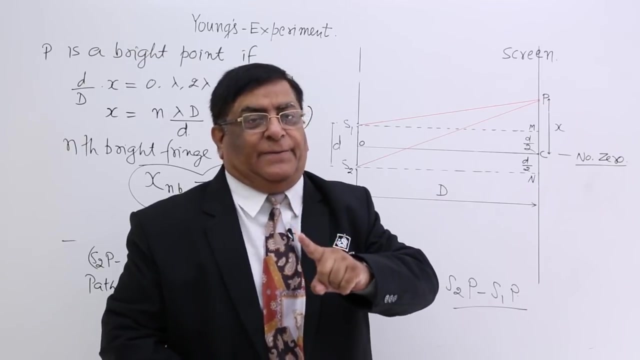 will be the 17th bright fringe. In the previous lecture we have seen the fringes will be alternate: bright, dark, bright, dark, bright, dark. This is central bright. After this central bright, there will be a dark, Then there will be a bright. Why? Listen carefully Here, what is? 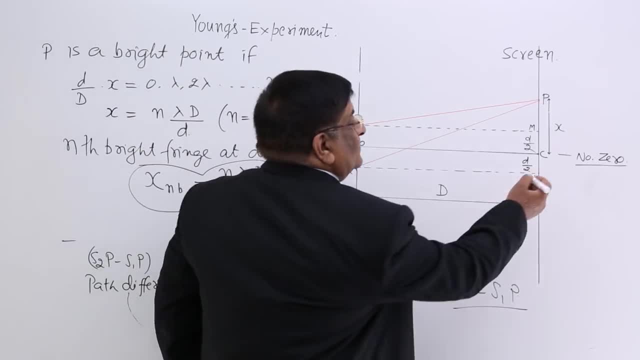 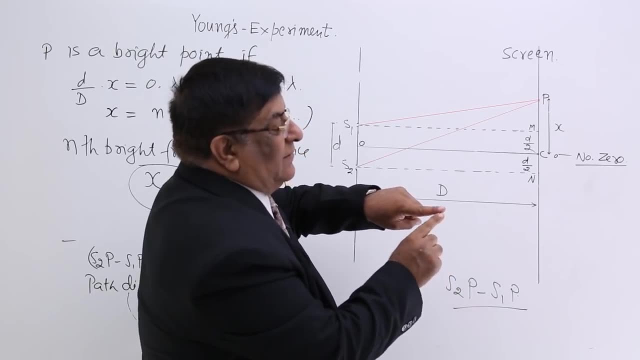 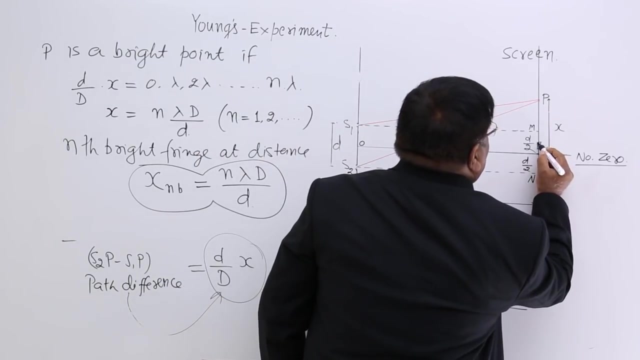 the difference of the path 0.. When we move them little up, how much is the difference of the path Lambda by 2.. When it is lambda by 2, what will be the fringe here? Answer: dark Again. move up the difference. 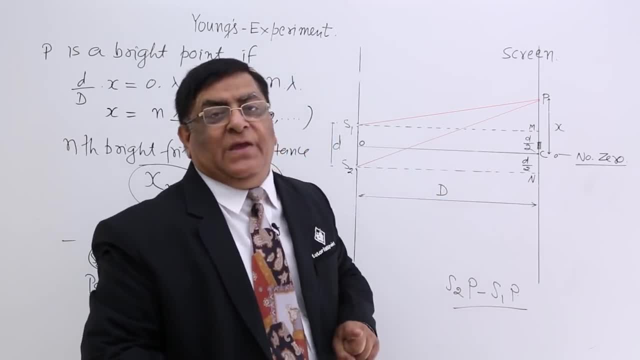 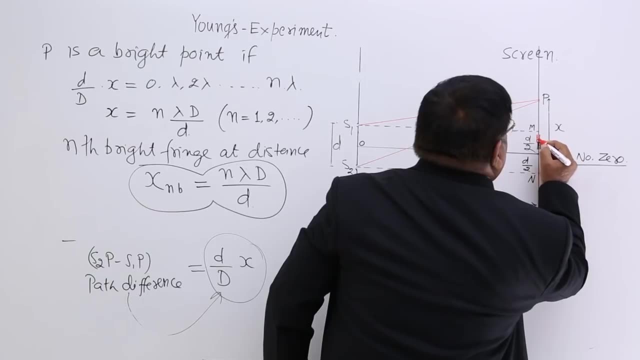 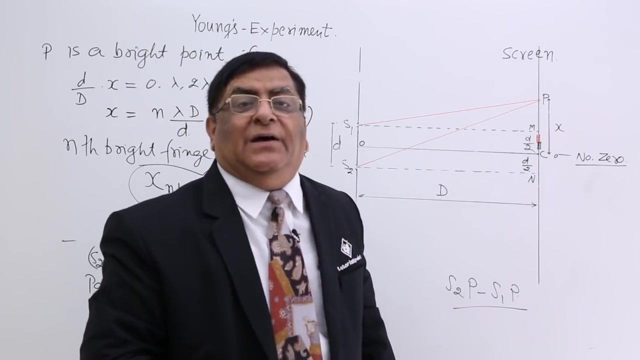 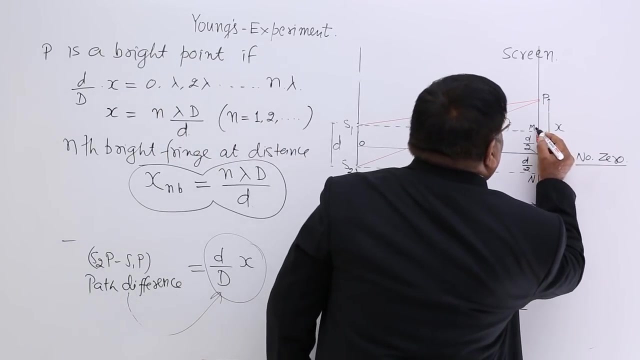 has increased and now it has become lambda. If it has become lambda, then what we get here? A bright fringe here. Move further. the difference has increased to 3 by 2 lambda, which is a odd multiple of lambda by 2. Then the fringe will be again a dark one After that move. 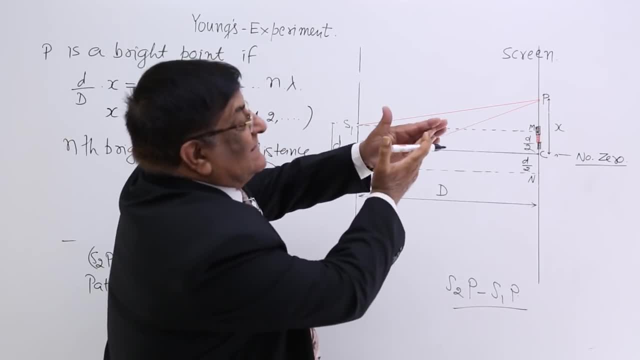 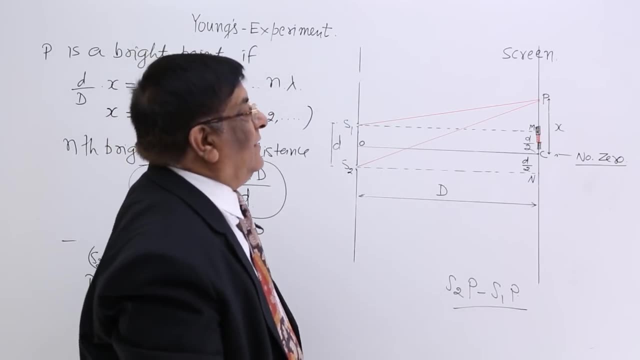 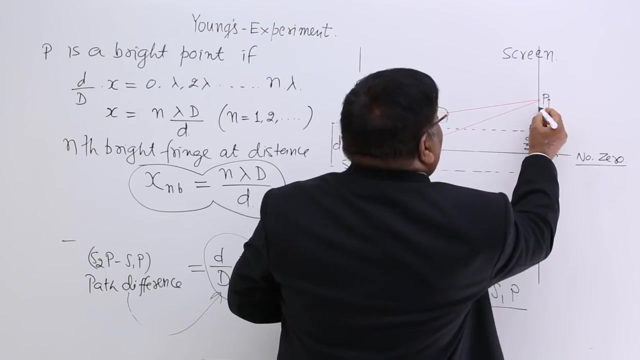 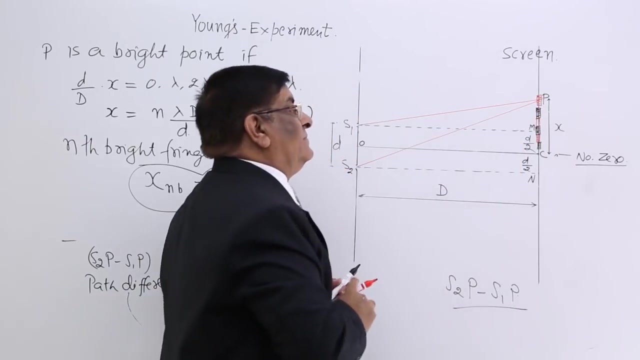 further. the difference goes on increasing, increasing, increasing. Then the difference will be, say, 2 lambda and it will be a bright fringe. In this way we get bright, dark, bright, dark, alternate. So we are getting alternate fringes this way, The same downward, and this: 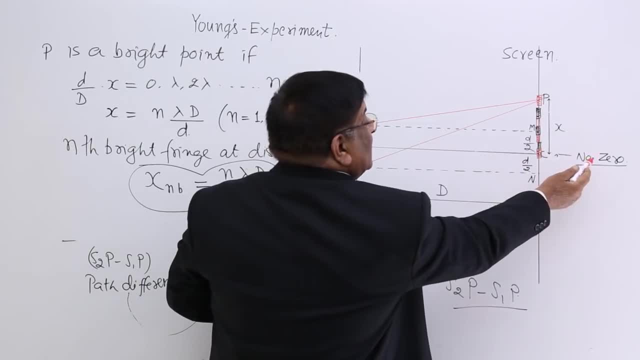 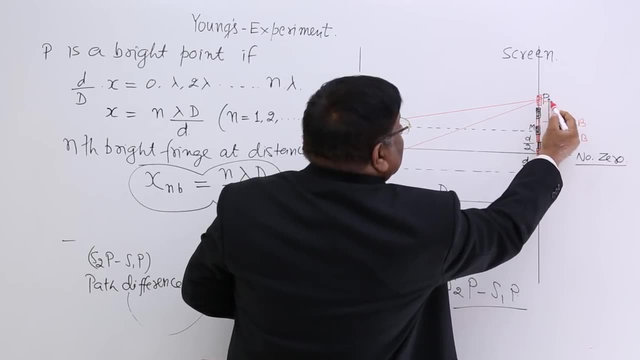 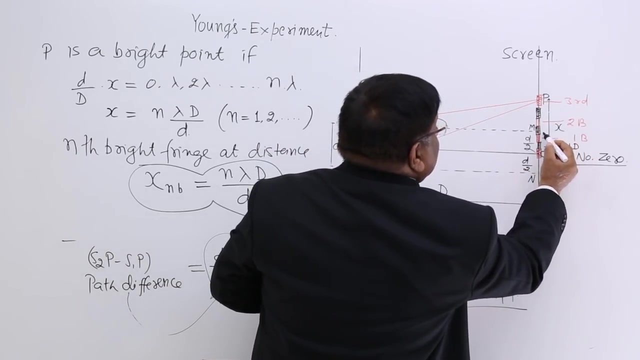 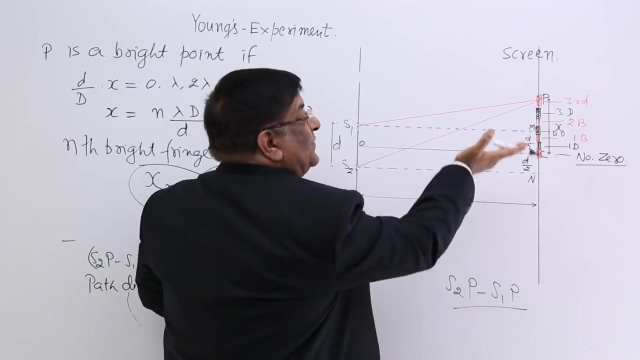 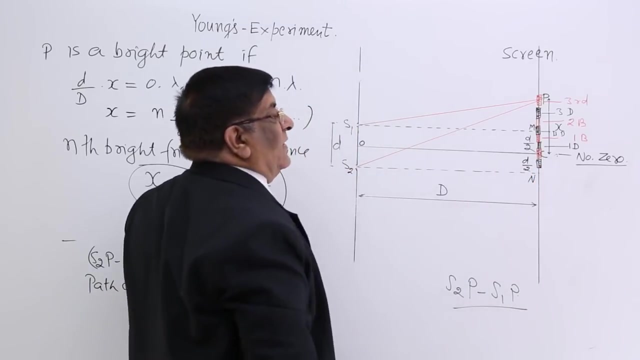 is central. This is number 0.. This is first bright, This is second bright, This is third bright. Like that, This will be first dark, This will be second dark, This will be third dark, and so on. Upside, Similarly, this is first dark downward. First bright downward. 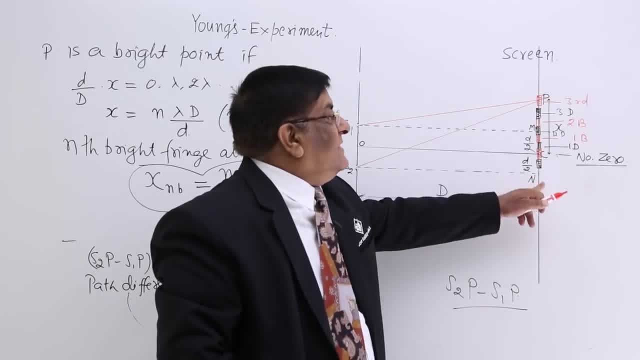 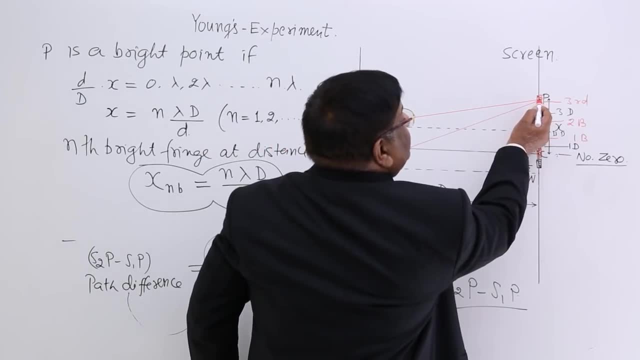 Second, bright downward. Third, bright downward. So there will be a series here. There will be a series here. So what is the distance of the fringes? 0.. What is the distance of the fringes, The distance of this, If I ask you that this is, leave this number 0.. After that, if this: 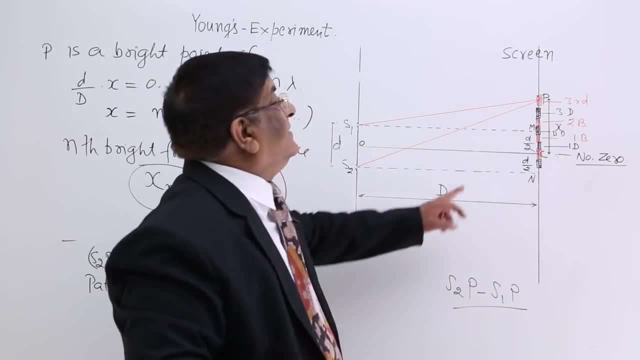 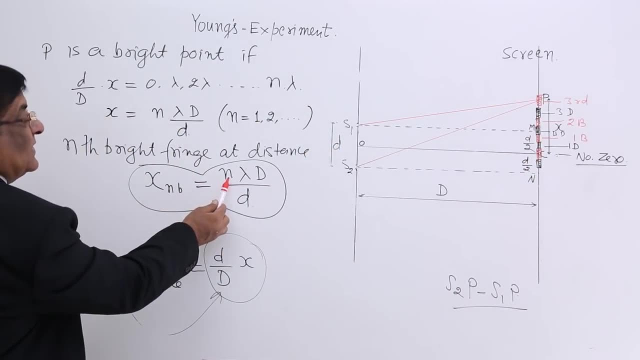 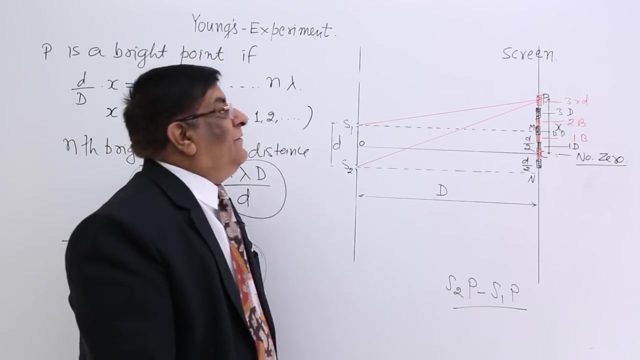 is the say 7th bright fringe. So what is the value of X? What will you do? You will put here 7.. Then lambda D by D. That gives you the distance. If I ask you, what is the distance from the centre bright? 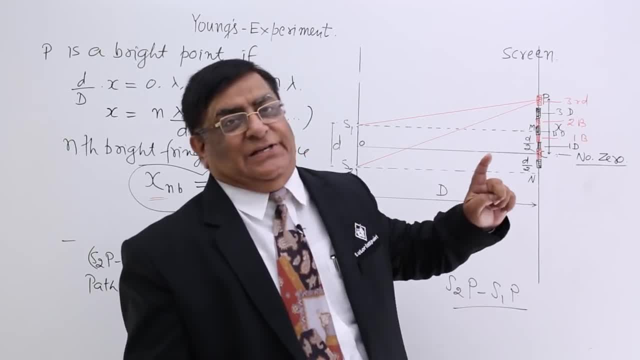 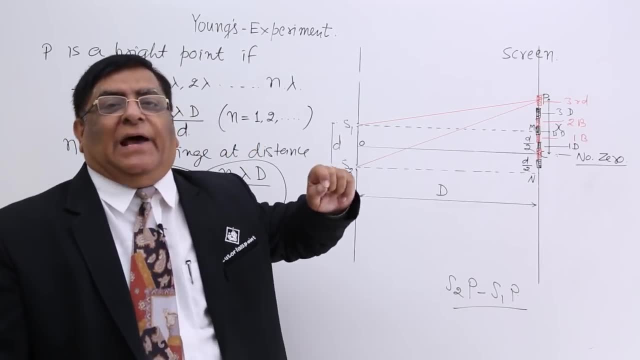 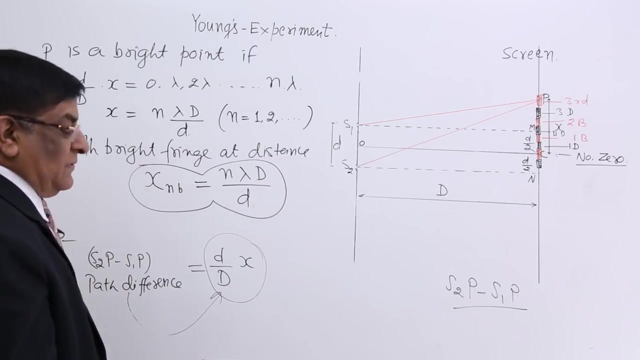 9. the distance of 9th dark fringe: 9th dark fringe. so you will take the formula of dark and put there 9. we will make that formula here. we have got the formula for bright fringe x. now we will see what is the formula for dark fringe. condition for this is condition for bright. 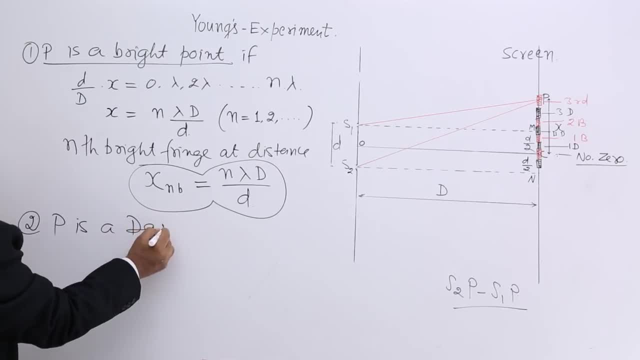 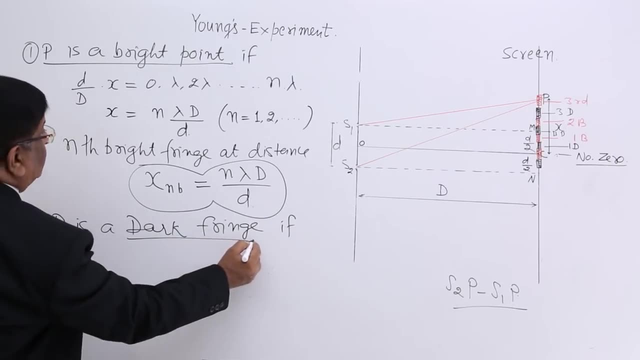 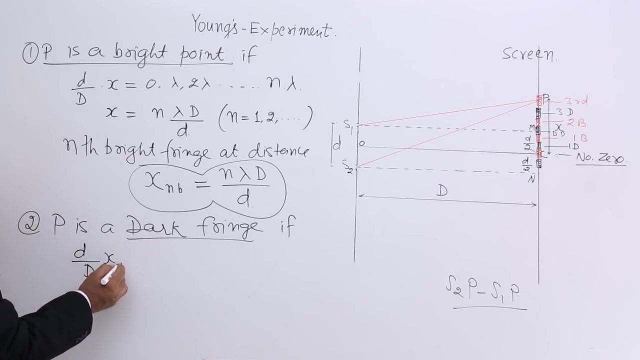 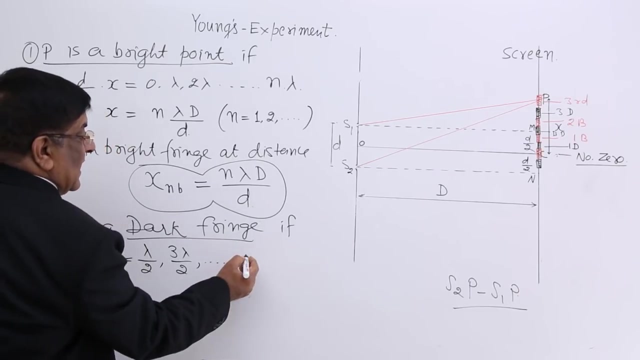 now, p is a dark point. if dark, bright, if path difference d by dx is equal to this path difference, it starts from lambda by 2, 3, lambda by 2, and this is n we want for the first we want there should be first. so we will write n: 2, n minus 1, lambda. 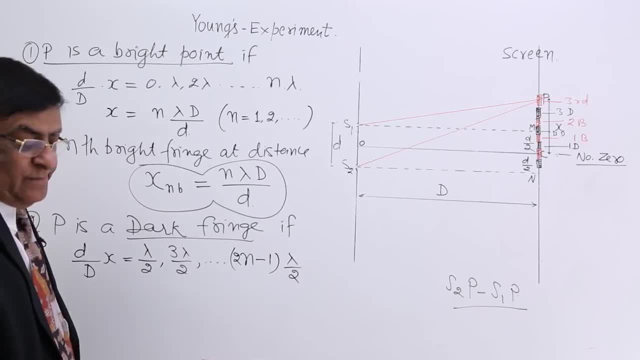 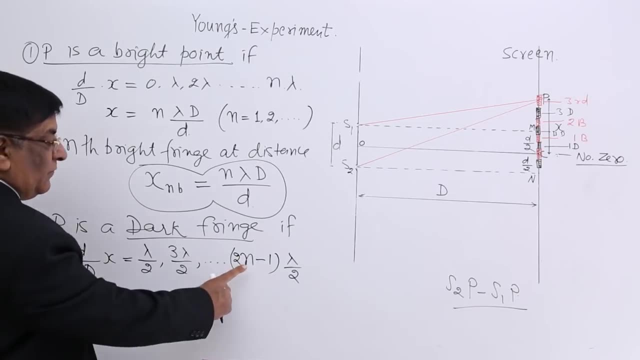 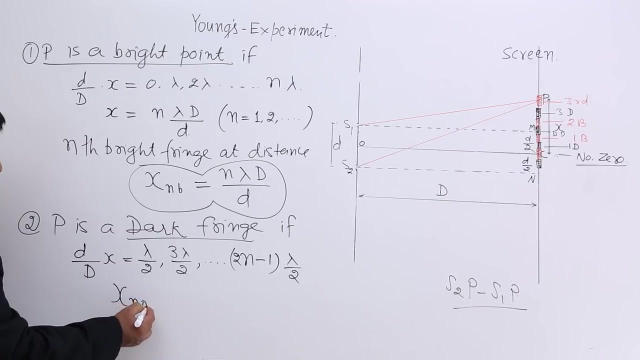 by 2. this is the general formula. so for the first brain it should come lambda by 2. put here 1. so if you put here 1, this is 2 minus 1, lambda by 2. that is the first fringe. so x for nth dark fringe this: 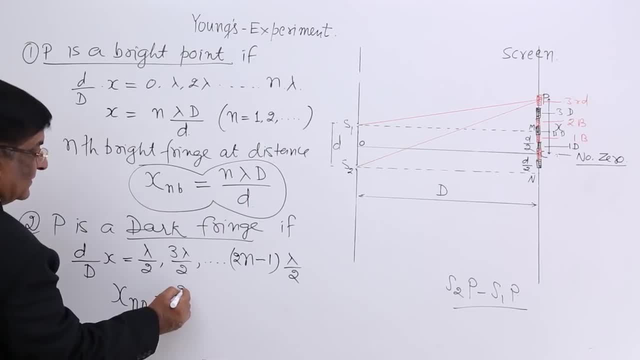 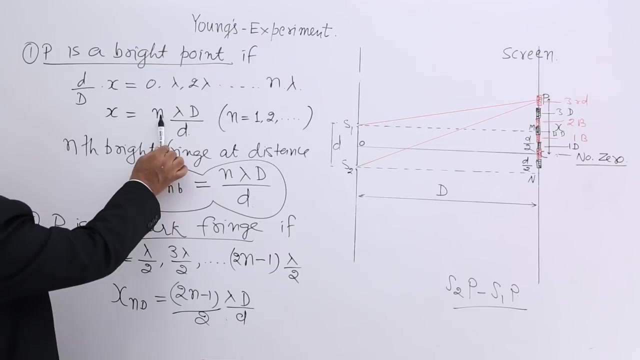 is equal to transfer this to on that side. so this will be 2n minus 1. lambda d by d and here 2. this You can say this way: lambda d by d, lambda d by d. This is n. 1,, 2, 3, 4.. This is what. 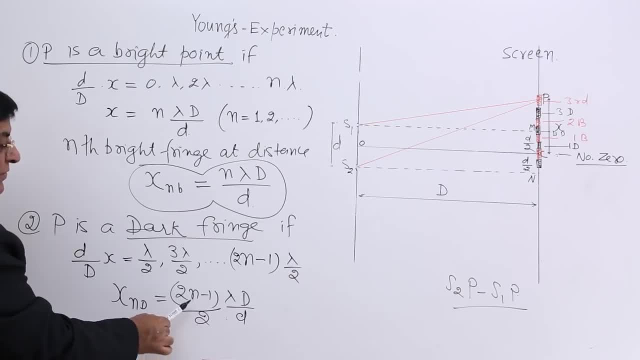 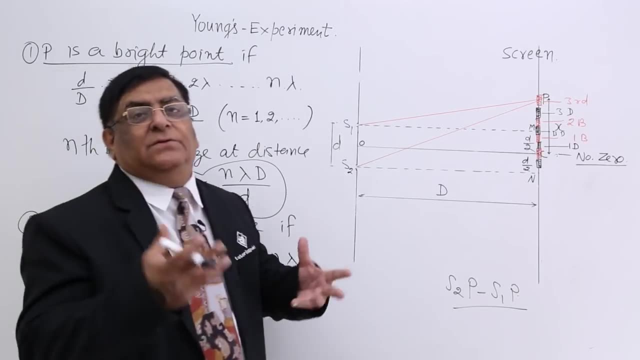 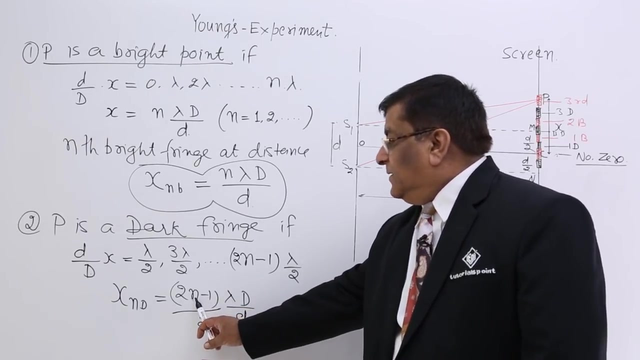 When you place it 1, then it is 1 by 2, then it is 3 by 2, then it is 5 by 2, like that. Now this is x. We start from central and put n is equal to 1,, n is equal to 1, and then 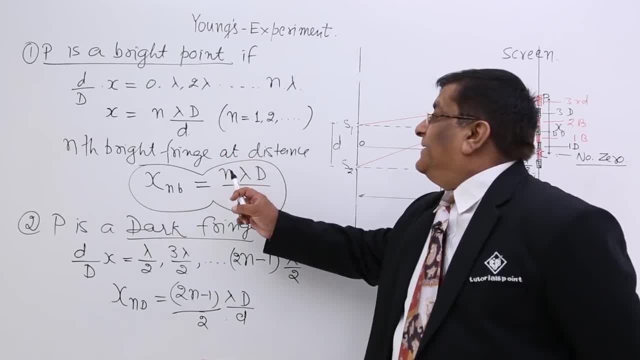 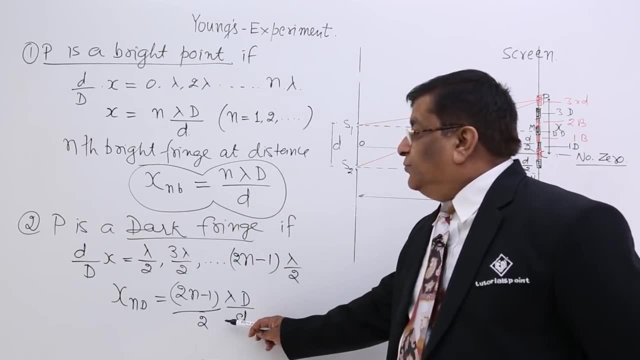 this will be lambda by 2.. If we put here n is equal to 1, this will be lambda. So which will come first? Naturally, lambda by 2- height come first, And lambda by 2- value of x will come first. 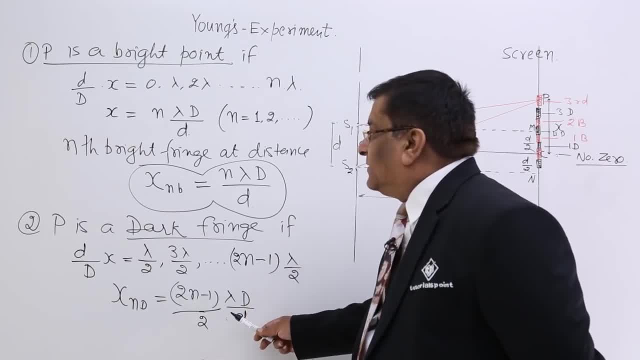 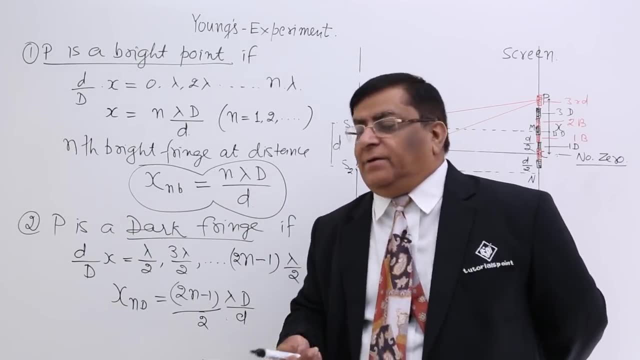 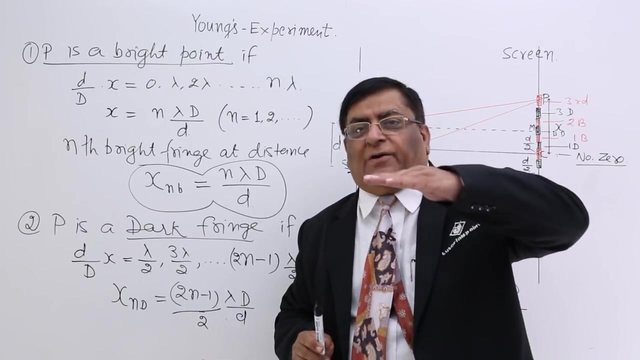 You keep on increasing. So first there will beondo be dark, then bright, then dark, then bright, then dark, then bright. and this is nth number distance. The distance of nth number of the fringe is given by this formula, and this is: 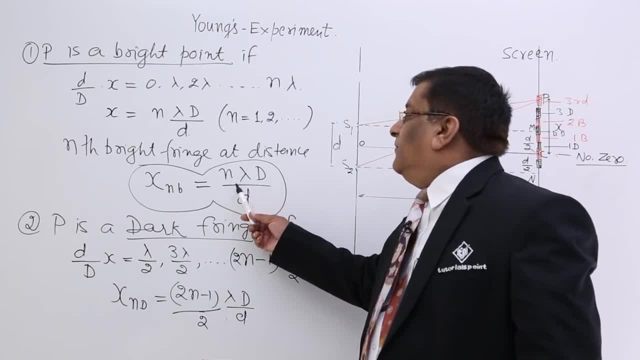 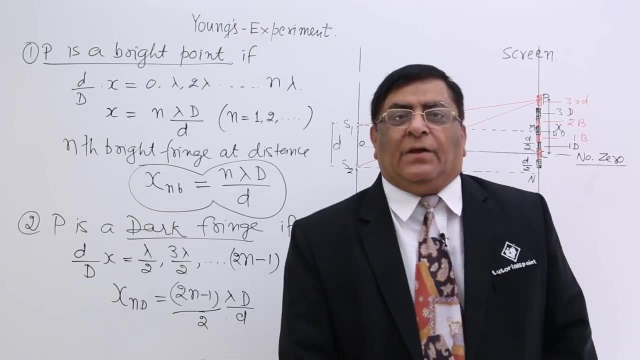 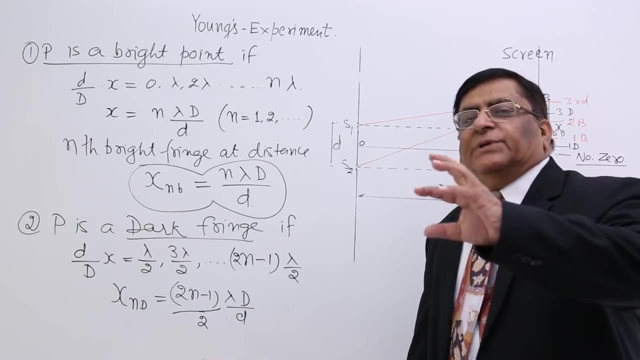 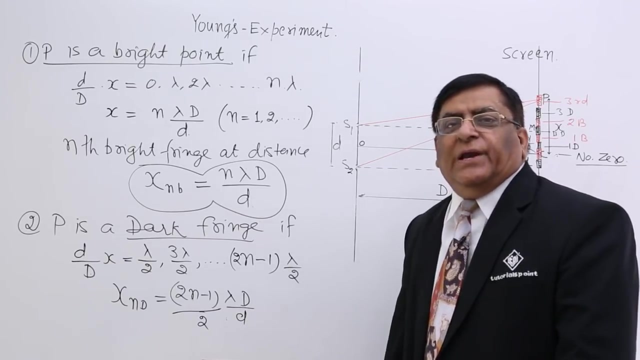 multiple of lambda by 2, this is multiple of integral lambda. So here we get it this way. So this experiment was shown by Young and it was shown in the lab. Once it is observed in the lab, then there was no need of proof. That was the proof itself that fringes are. 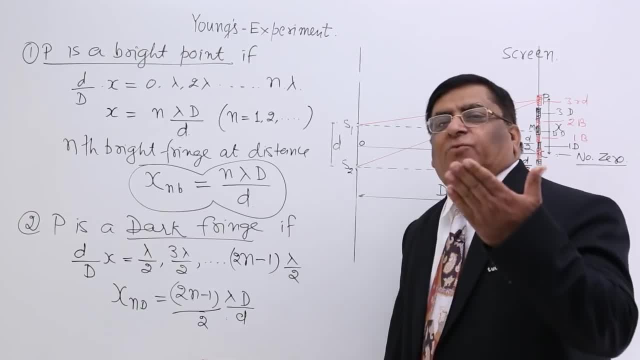 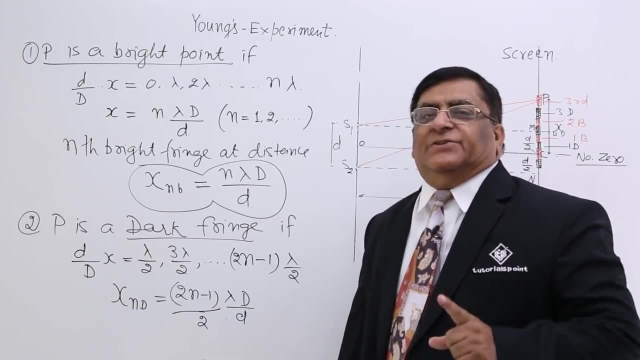 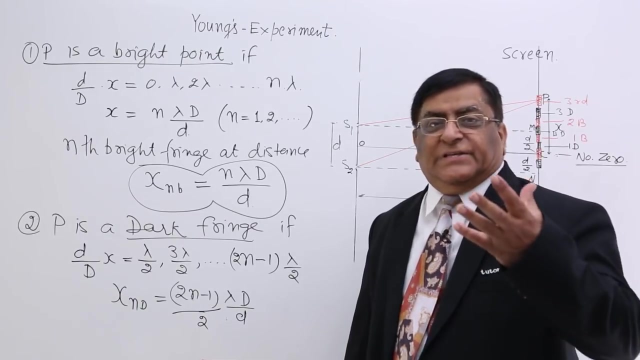 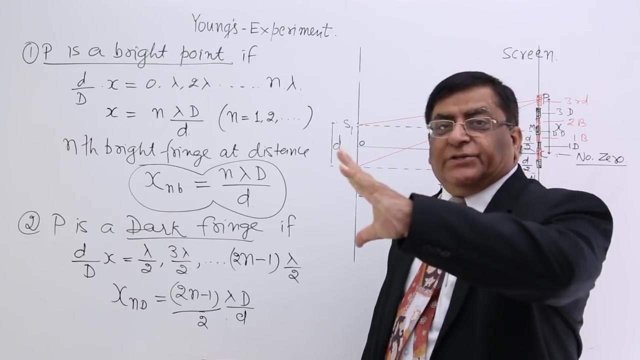 made. So now I will show you how to explain. the explanation was already done by Heijen. So with this experiment it was proved that Heijen's wave theory was correct. and that was a big thing. in physics, The complete theory of Newton, that is corpuscular theory, that light goes. 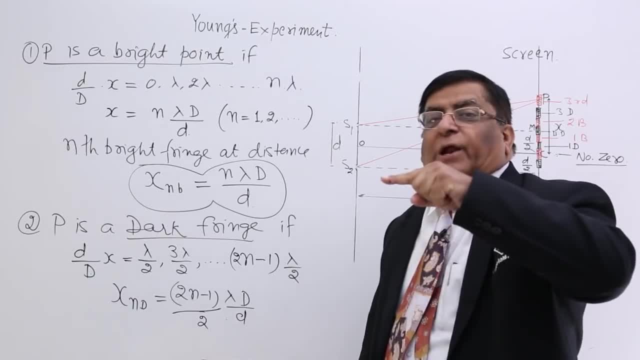 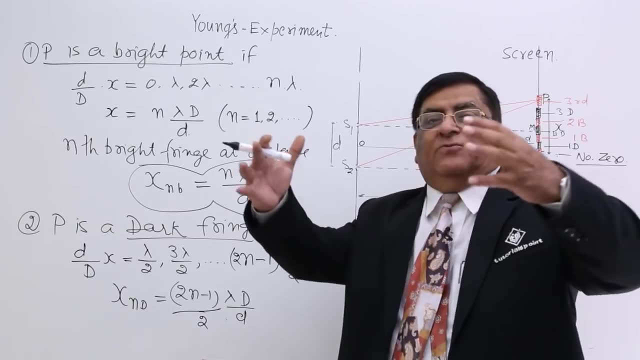 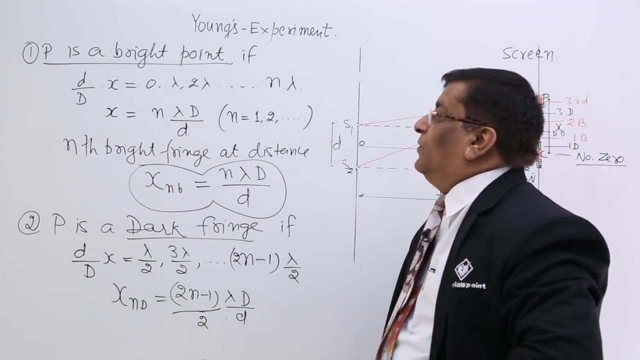 in corpuscles, which goes in a straight line like a bullet that was rejected. Now how the light was going: It spreads like waves of water in crests and troughs like this. So this was how it was established by this experiment. With this experiment, 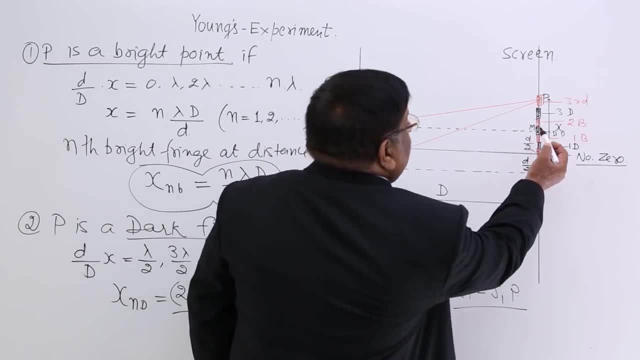 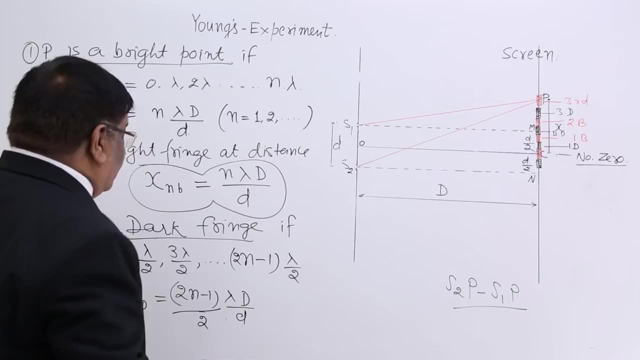 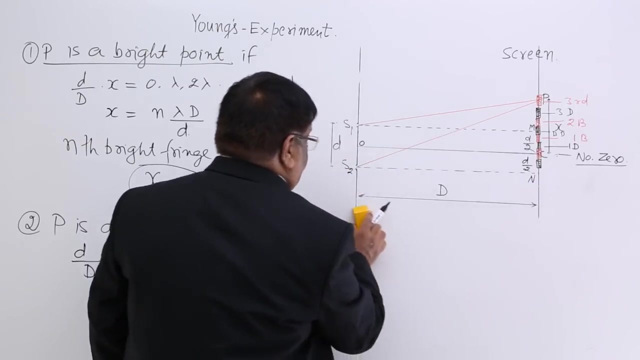 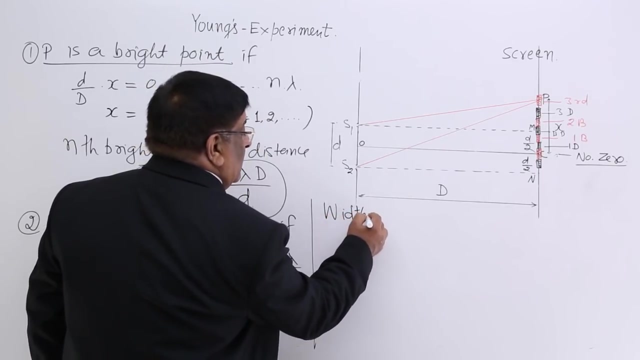 we are also able to find out the width of bright and dark fringe. To find out the width of bright and dark fringe, first we define that how we understand what is meaning of the width. So we will write here formula: width of light fringe is equal to n. 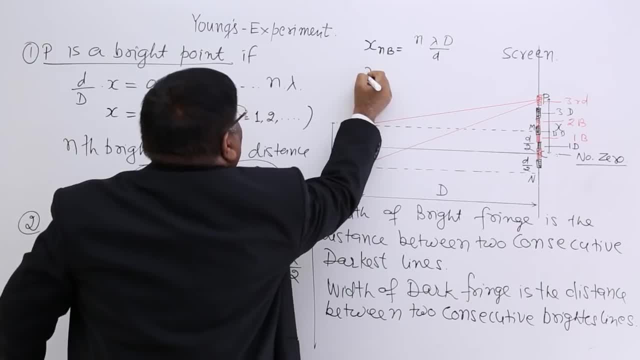 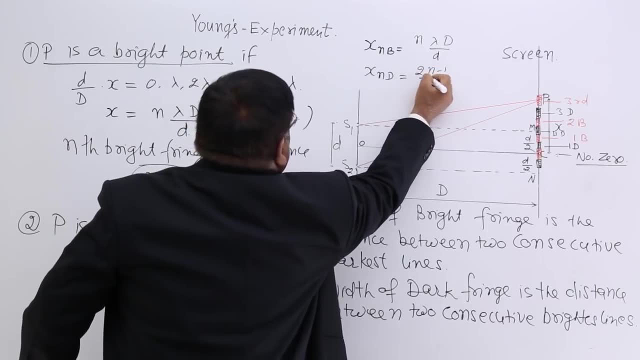 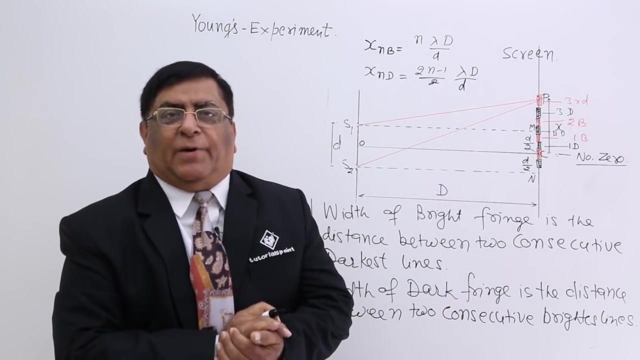 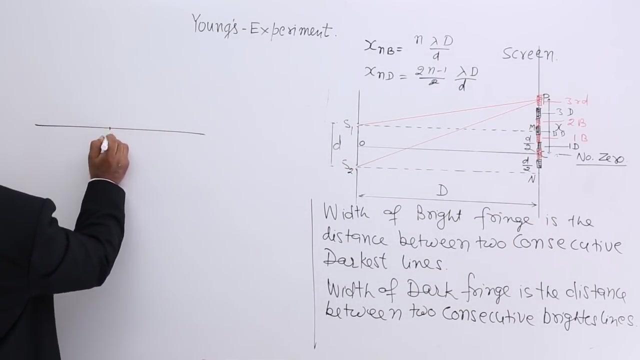 lambda d by d. X for nth fringe, dark fringe, is equal to 2n minus 1 upon 2. lambda d by d, We make a graph for the brightness versus this distance. Here is the point C, central point, and height will show. 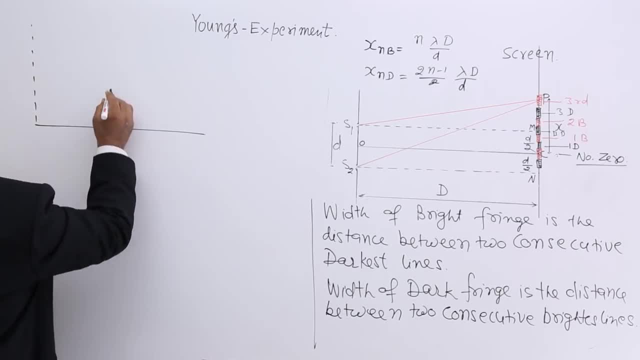 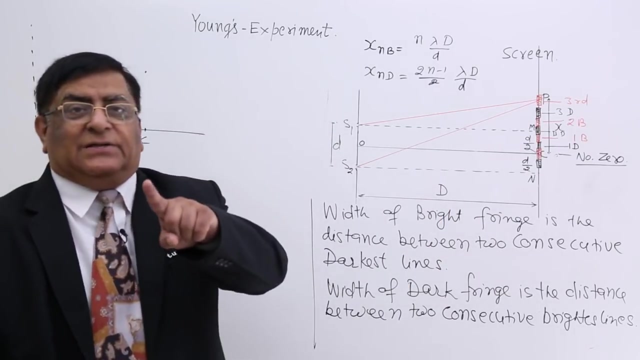 the brightness. At point C the brightness is maximum. Now I will make it little bit here. This is point C and here the brightness is maximum. If I go a little away from this, then what will happen to brightness? Answer: the brightness will decrease. 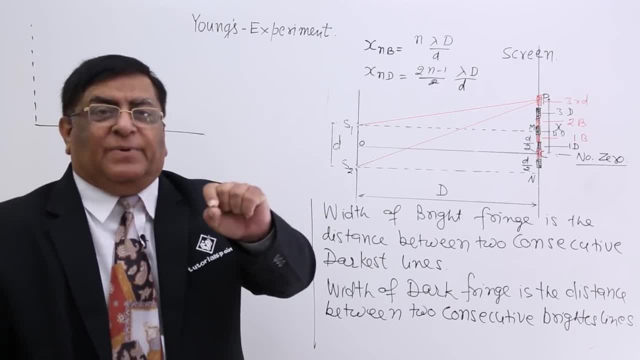 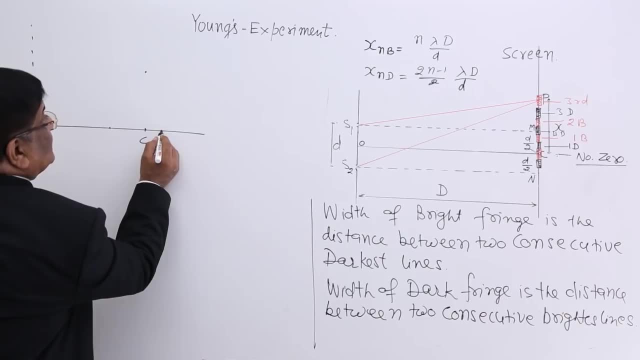 because the difference will not be exactly 0. It will be slightly different, But it is not lambda by 2.. So when the first distance is 1, this is half lambda d by d. This is the distance half lambda d by d. 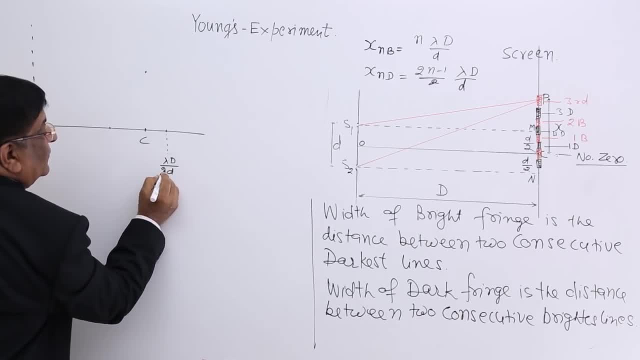 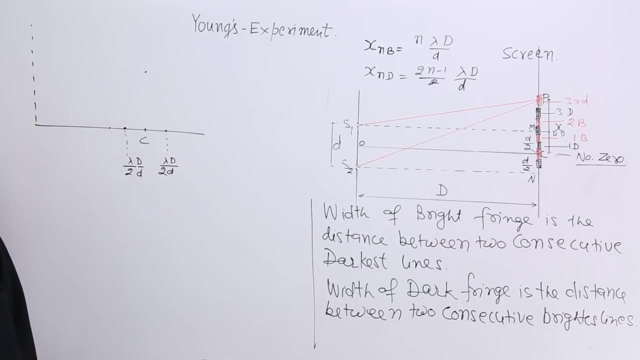 Lambda: d by d, half. So this will be the darkest point on this side, and this will be the darkest point on this side. What is the distance? Lambda by 2, d by d. Now, this is dark. This is maximum bright. What about this point? 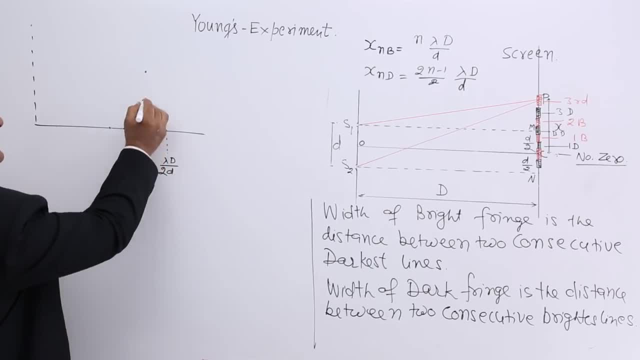 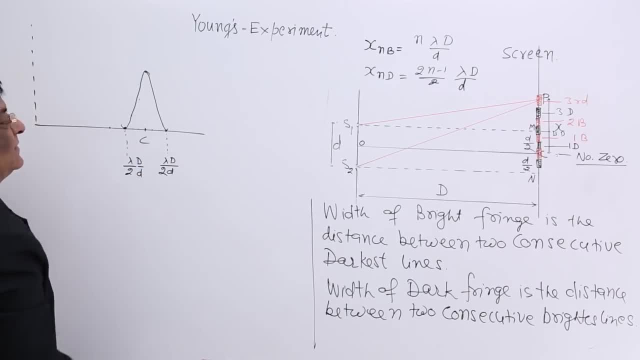 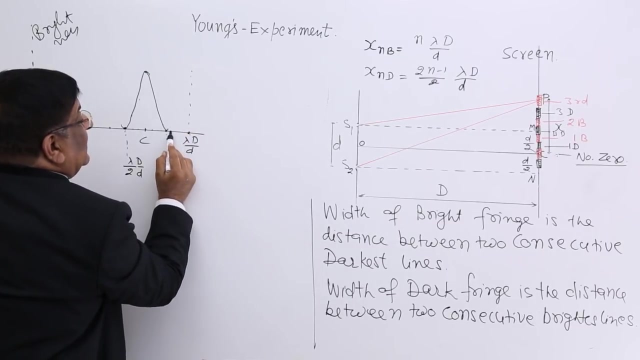 So then, where is the first bright, first bright, first bright, first: lambda d by d. this is half lambda d by d, and this is one lambda d by d, lambda d by d. this is again a very bright point, and here brightness is much. this is brightness. so from this point, brightness start increasing, increasing, increasing. 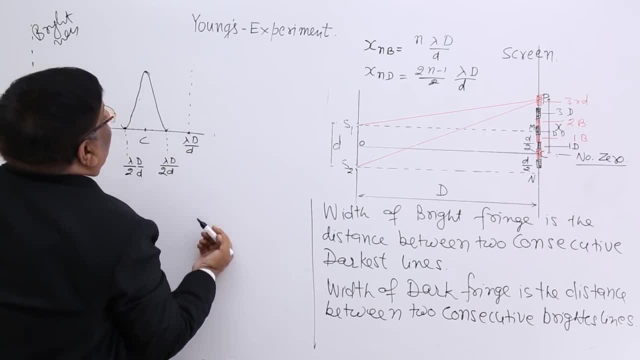 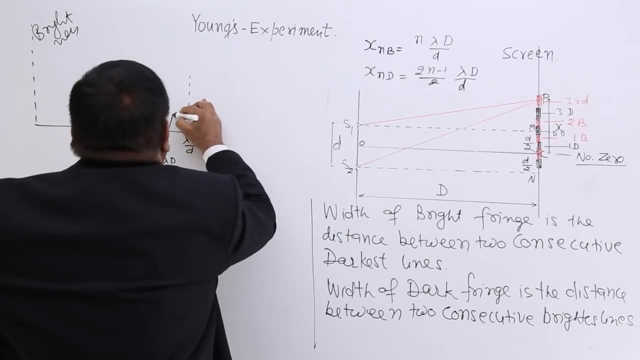 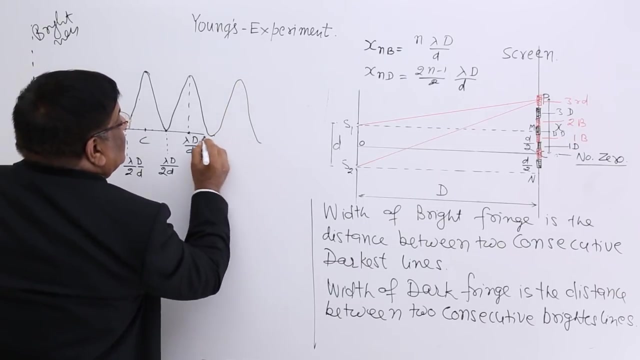 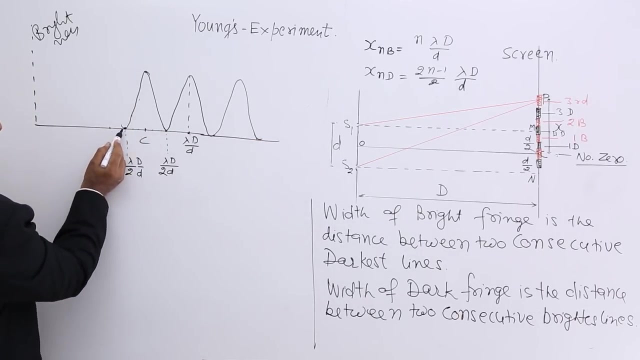 maximum, decreasing, decreasing, decreasing, minimum. so we make a graph here which is like this again: it is like this, similarly on this side: half lambda. then this is one lambda at one lambda. it is maximum, again at half lambda. it is minimum, again at half lambda. maximum, again at half lambda, it. 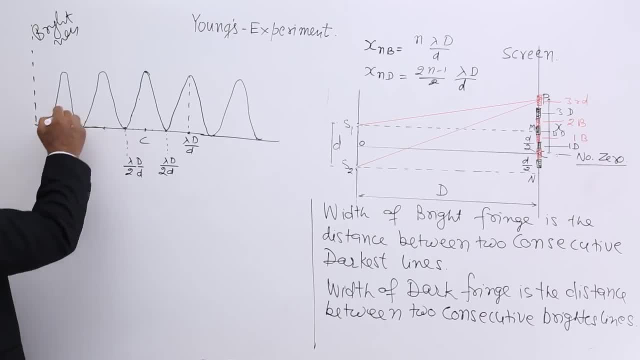 is minimum. so this is our brightness versus distance, distance from the central point. these are all equal brightness and these are all equal distance. so this has become a symbol, a trademark for interference fringes, now brightness, and what is this point? dark, dark. this point is how much. 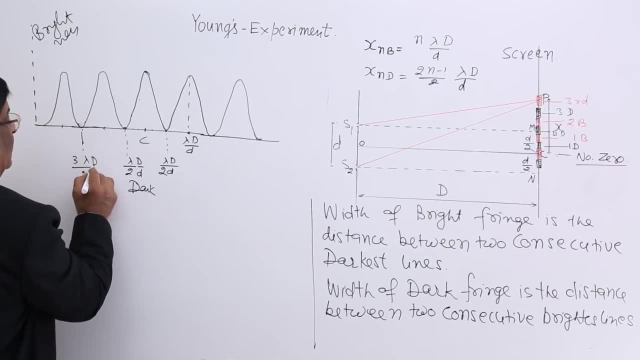 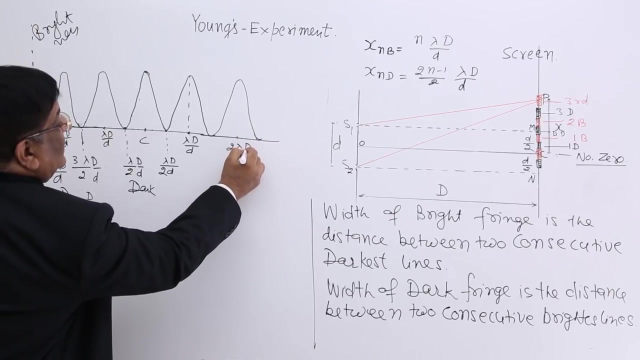 looks right. つ. lambda by two, d by d, this is five. lambda lambda. and so this is dark, this is dark. so this is dark, this is dark, this is bright. how much is this lambda divided? this is right. one to los Angeles derby, this is quite too. and business three by two, and to the three, two by two. 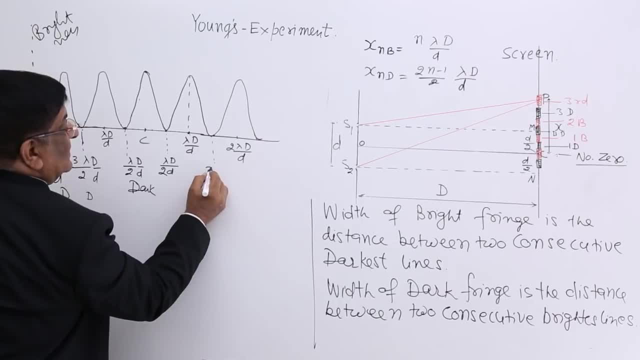 lambda divide. this is bright one. this two and to the three, two. this is bright one. lambda divide, this is bright one. and to the three, two. and to the three: two. has three by two, less than 하게ポリスト k. microsympathetic AB cloth fiftyragic transpose прирcam. 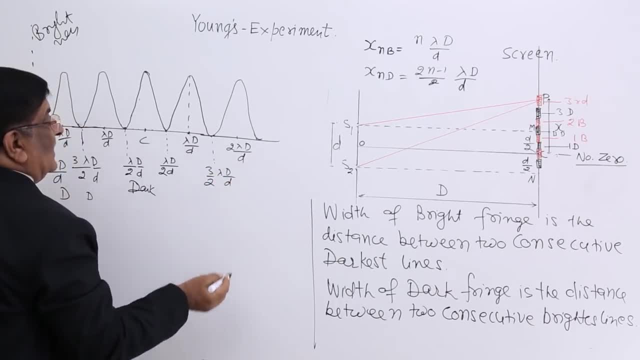 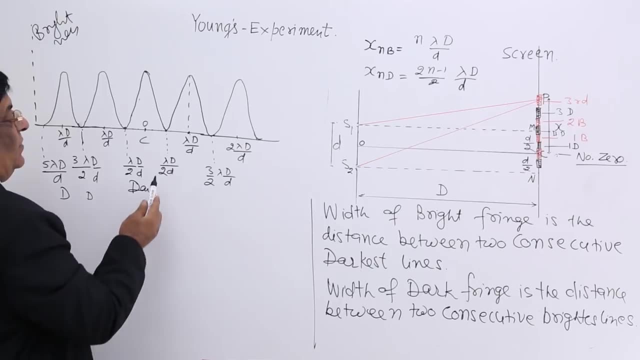 driver. to me this is right. figure span in this means this should not be one drugs, the two sieve to display lambda d by d, See every half lambda. there is a difference Here. the difference is 0.. After half lambda, it is dark Again. after half lambda, this is bright Again after half. 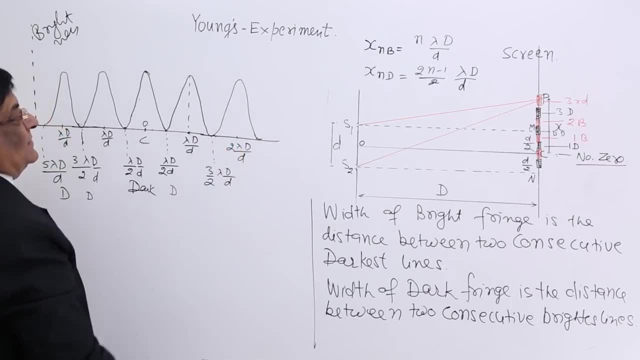 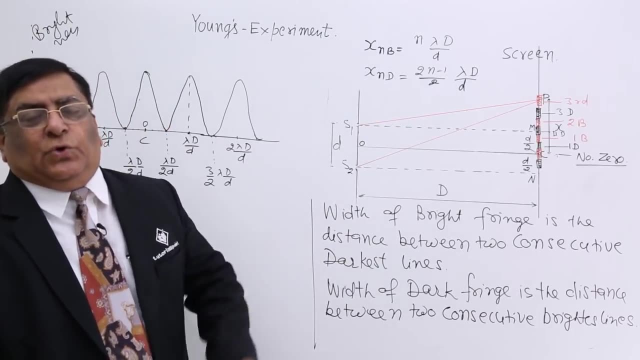 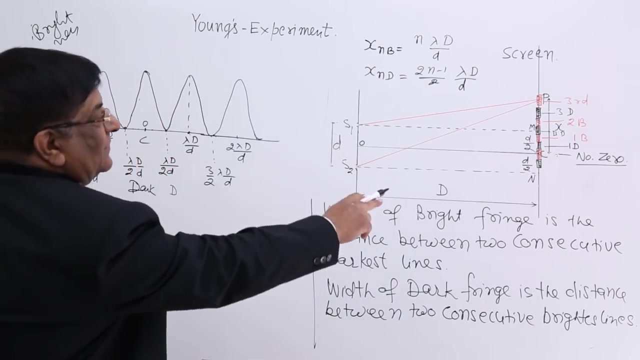 lambda, it is dark. Again after half lambda, it is bright. That is what is said by our calculation and that is what we see practically. So that means wave theory is calculating correctly and this is the interference fringes. This was shown by Young's experiment and 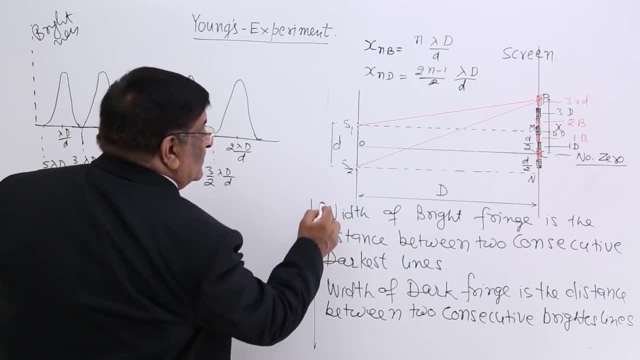 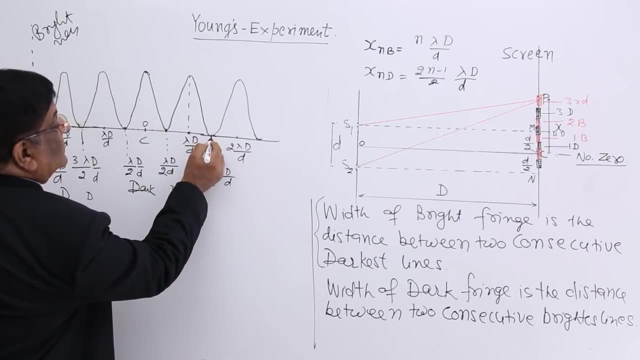 now we have come to the topic: width, Width of the bright fringe. from dark to dark, from this dark to next dark, This is width of the bright fringe Here. this distance is this much minus this distance, If you do this, minus 3 by 2 minus. 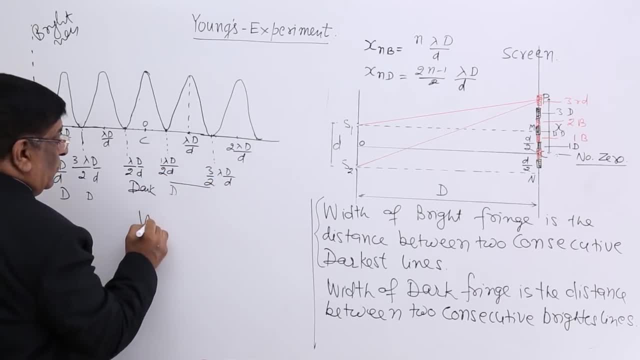 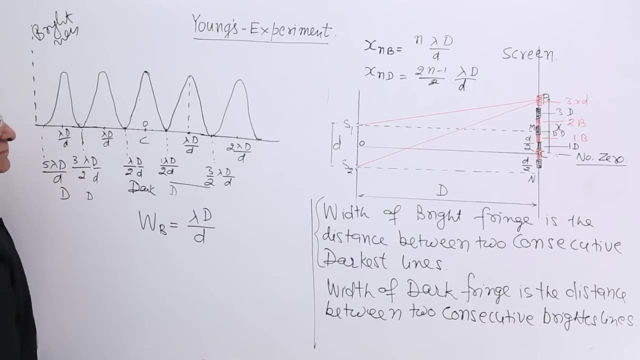 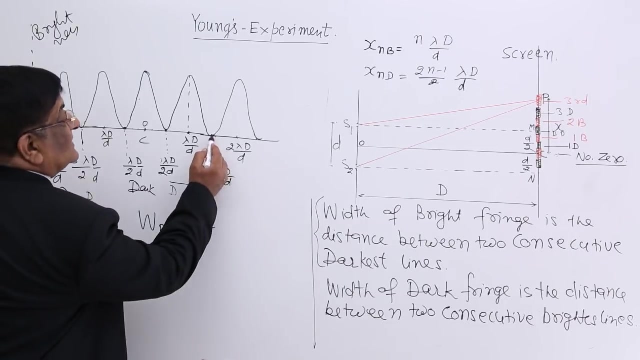 1 by 2 is equal to 1.. So, width of the bright fringe: we get as lambda d by d Again. width of the dark fringe: Where is the dark fringe? This is the dark most point. This point is the bright most point. This point is the light most point. This point is the dark most point. 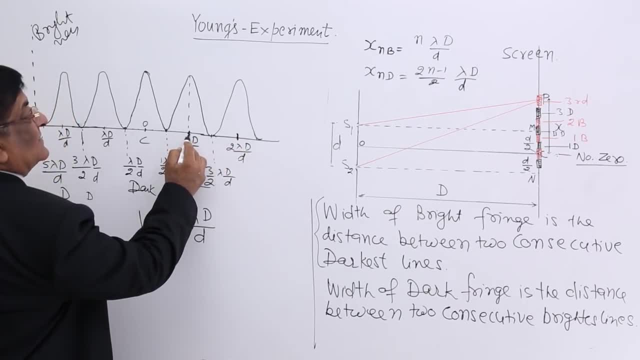 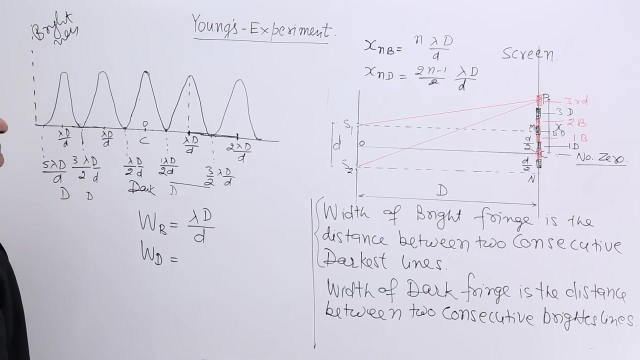 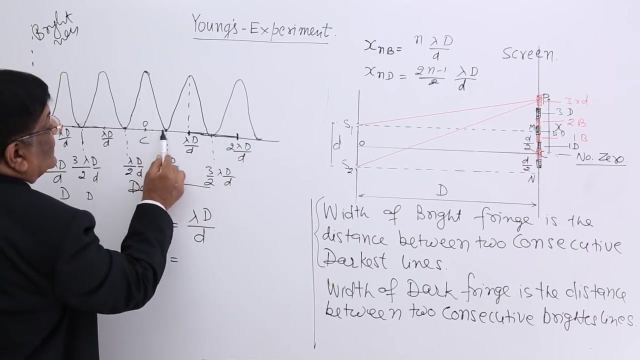 brightest line, this is the brightest, next brightest line and brightness decrease, decrease, decrease darkest and brightness again increase. so this is again maximum dark and this is taken as width of the dark fringe, bright to bright. and how much? this is 2 lambda d by d distance minus lambda d by d distance. this is equal to, again, lambda d by d. you can do. 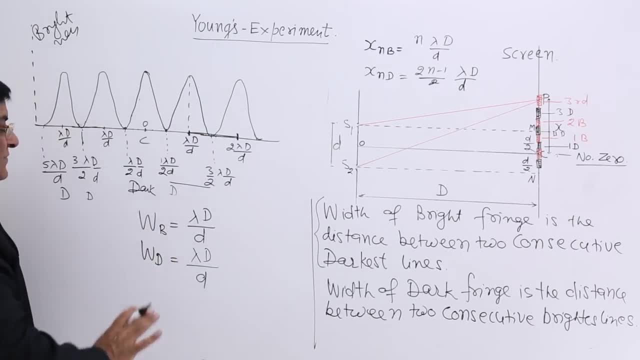 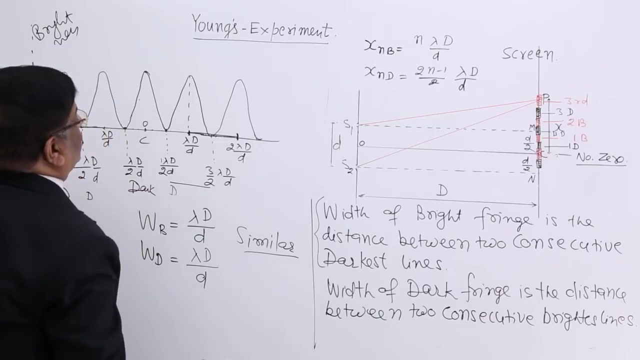 this minus here, here, here, anywhere, it will come same. so width of the dark fringe, lambda d by d. width of the bright fringe, lambda d by d. that means their widths are similar. okay, what is width of the central bright fringe? central bright fringe half lambda here, half. 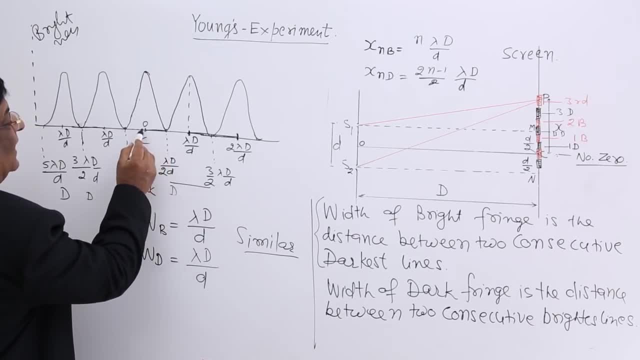 lambda here. so half lambda here, half lambda here. and what is this width? that is again one lambda width of the central fringe. this is equal to, again, half lambda by 2 multiplied by 2. lambda by 2 multiplied by 2, that is lambda d by d. so we find whether it. 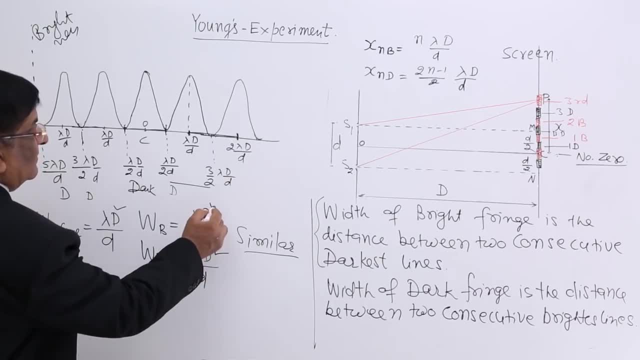 is central fringe, whether it is dark fringe, whether it is bright fringe, whether it is dark fringe, whether it is bright fringe, if there is some, load your floor, because if you basically imagine this, dense لا, you are depending on the color with the chromatic wall surface. once again, the area x is 0. i amosing this into a square.